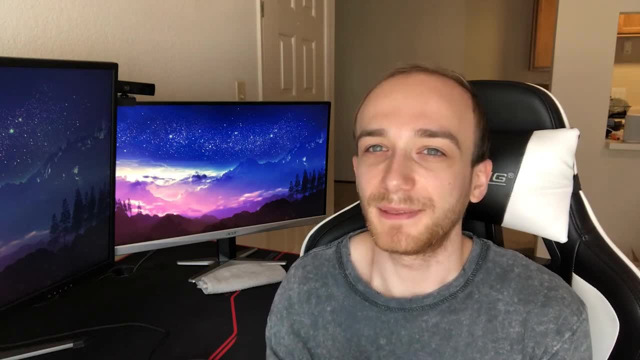 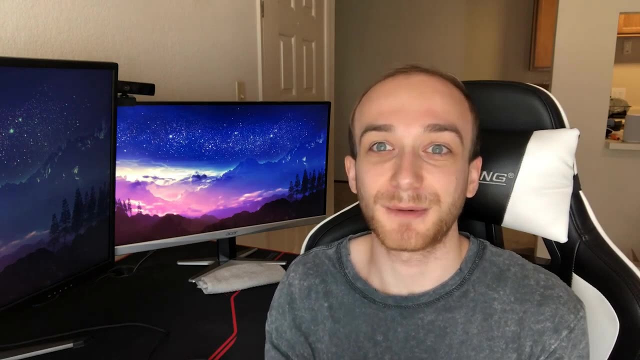 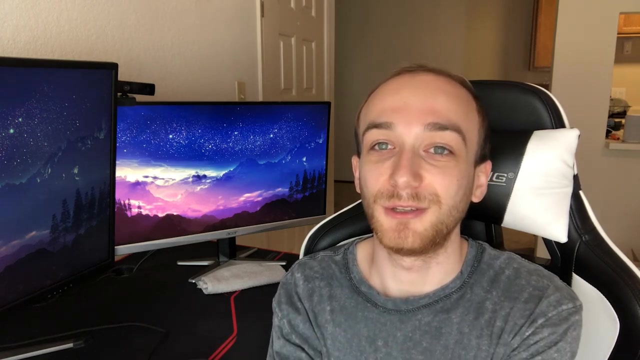 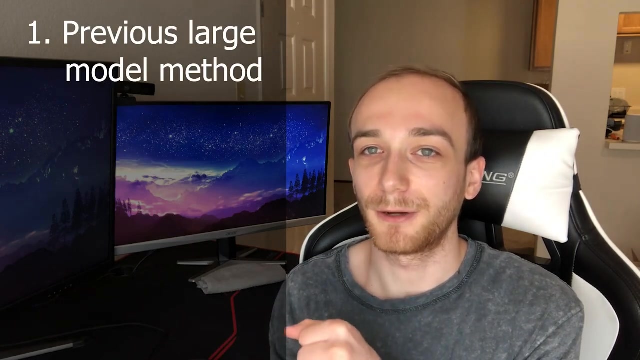 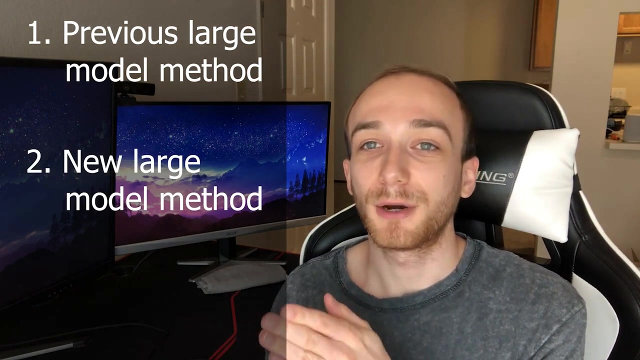 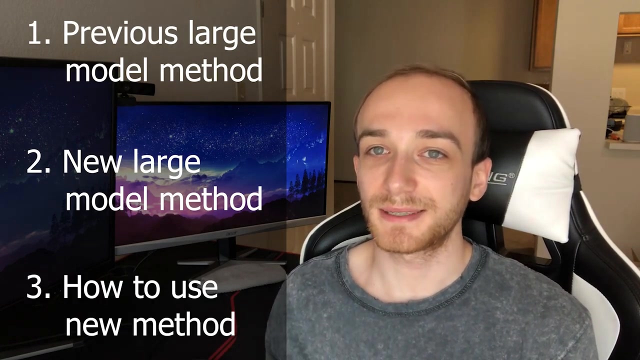 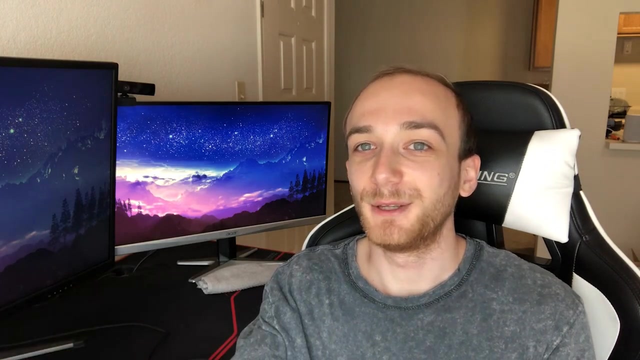 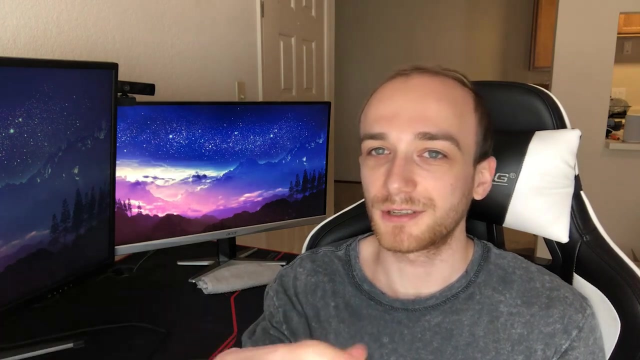 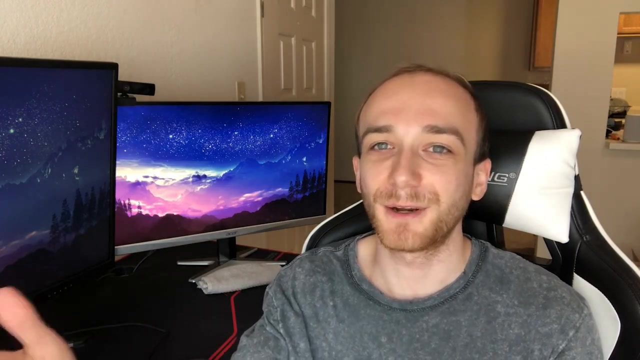 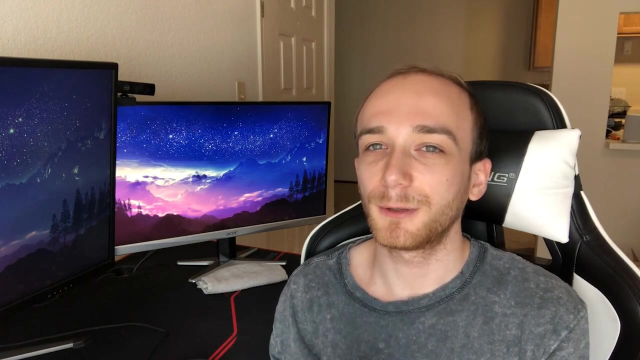 I like to just read core machine learning stuff really the theory but this is this is a systems problem really with a sort of machine learning wrapping over it so I wasn't thinking I would like it as much as I really ended up liking it because it's just it's it's incredible what they've achieved in this paper so that's why I'm really excited to share it with you all today. Specifically I'm going to be talking about first the previous method that we were using to do this sort of parallel computation and then I'm going to move into talking about this new method. What's different specifically what are the different components of it and how it works and then lastly I want to wrap up by talking a little bit about how you can actually get your hands on this technology as soon as today because there are actually already a lot of libraries that are using this paper. Now if any of that is the type of thing you like to watch or listen to do consider subscribing to the channel. I talk about a whole lot of related content anything from research to my experiences at companies like Google and Amazon to doing research all sorts of reinforcement learning stuff all sorts of stuff so if you are interested in learning more about parallel computing I'll be happy to help you out. If you are interested it does help out the channel a lot and it does mean a lot to me but anyway without further ado let's first jump in to a little discussion on how we've 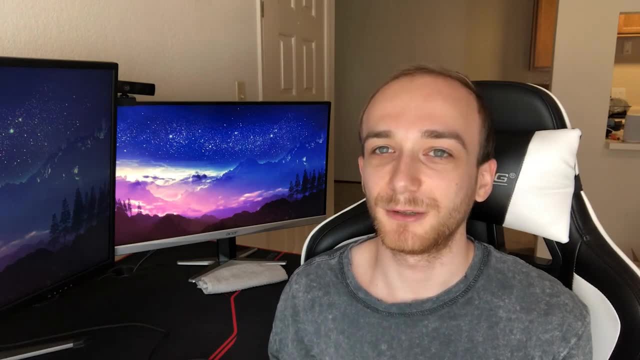 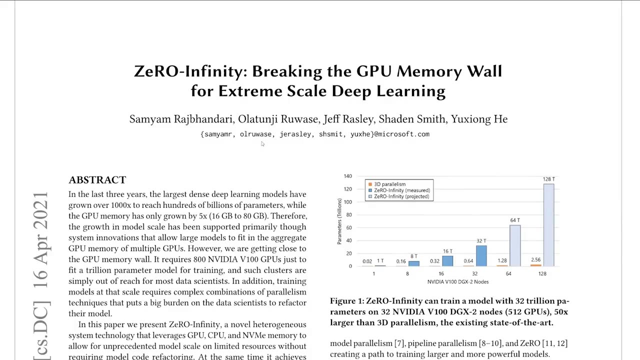 been handling this parallel machine learning data stuff up till now so that I can really set the stage for how we've progressed and what this new paper really brings to the table. Okay so here we 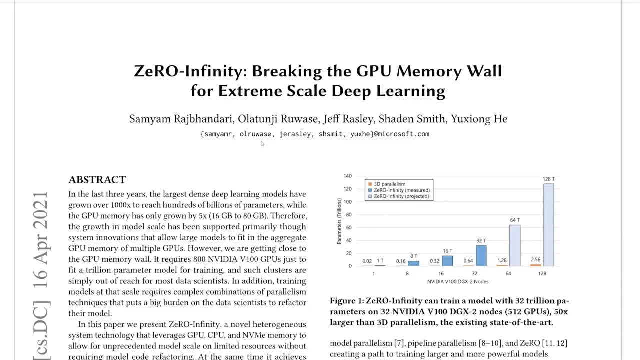 are in the paper I want to start off by talking about the setup here why this paper was so necessary and sort of what the motivation behind this was. If we look at the abstract we can see that within just the past three years model sizes have grown a thousand fold this is to reach hundreds of billions of parameters they're probably referring to GPT-3 right here although I think there are other models now that also reach that size which is crazy right 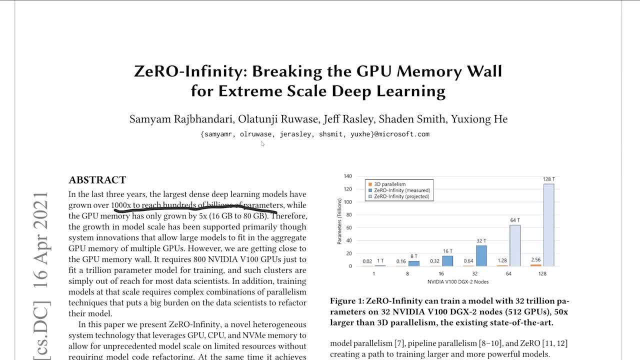 that is absolutely ridiculous GPU memory on the other hand has only grown roughly five times you know five times a thousand times clearly the scaling doesn't match up here so we essentially need new ways of accounting for this right now to change or what is the 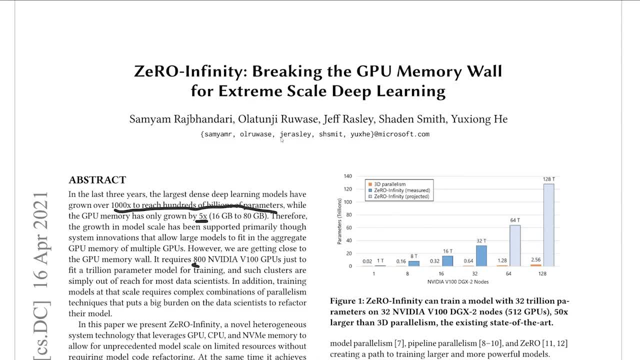 to train a trillion parameter model it takes 800 nvidia v100 GPUs and each of those GPUs are quite pricey it's a crazy amount right this clearly is is not scaling very well and something 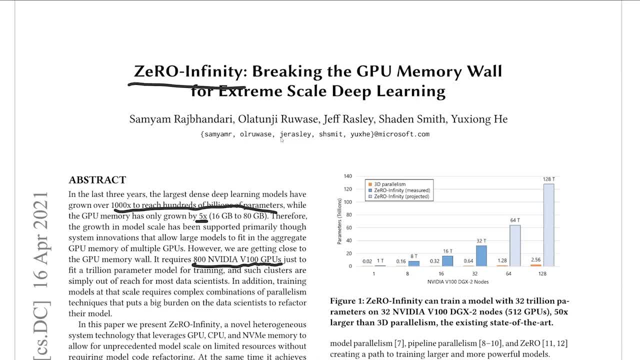 needs to be done about that and that is why we have zero infinity this paper and great name by the way breaking the GPU memory wall for extreme scale deep learning so that's sort of why this needs to happen so the method that was being used before let's go up here real quick was called 3d 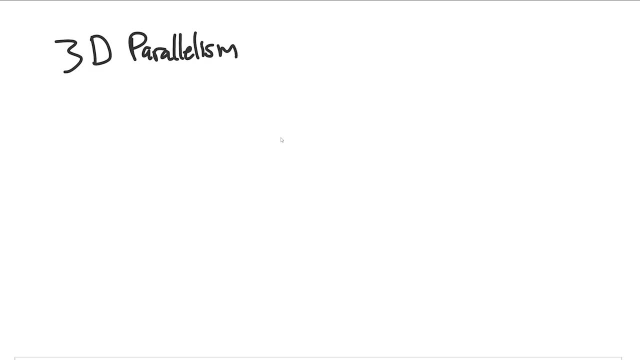 pair hopefully I spell this parallelism I think and essentially what this is is it's a method where you essentially break up your model into different pieces different tensor slices and you 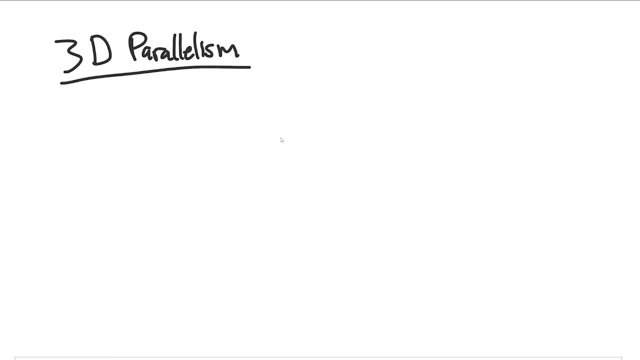 run those computations in parallel across different GPUs right so essentially all the parameters just sit on different GPUs and you do different computations on different GPUs it's fine right 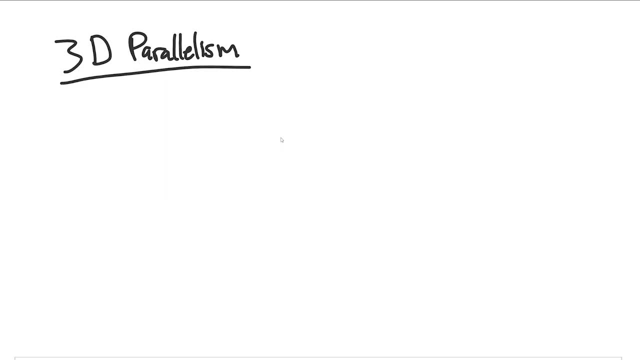 but once you take into account that thousand to five fold increased comparison well clearly we really are running out of GPU memory so we're not going to be able to do anything about that 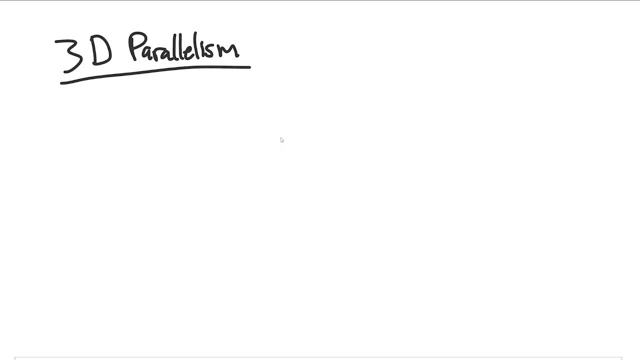 we need to do something about that so there's a few problems with 3d parallelism one is what I just mentioned right not enough enough enough GPU space that's a big one probably the biggest one 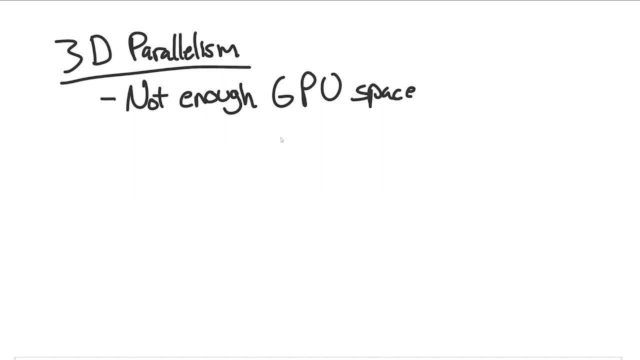 and and not only do we not have enough GPU space but sometimes when you're when you're making these models with 3d parallelism you have this sort of constraint you have to work in with the which is 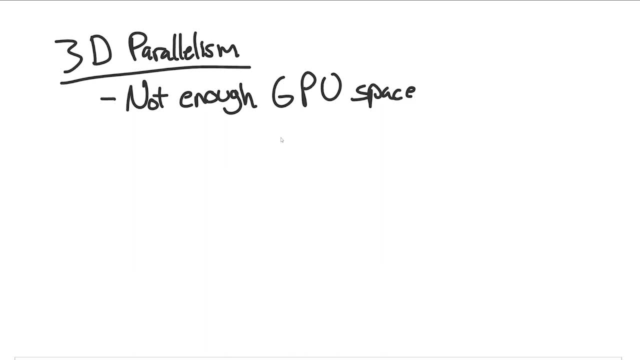 a single layer you have to work in with the which is the largest single layer in your model has to fit into a single GPU so if your single largest layer even though it's just a single layer is larger 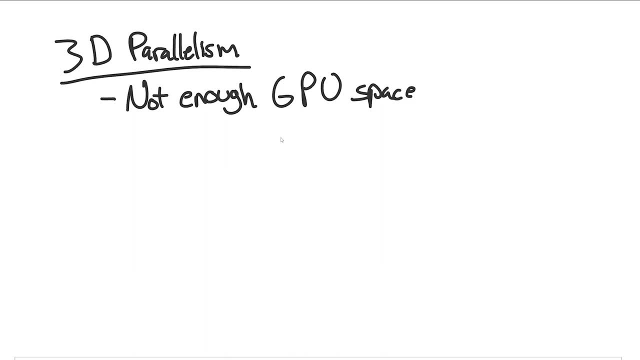 than the amount of space a single GPU has you actually can't run that model so it doesn't work 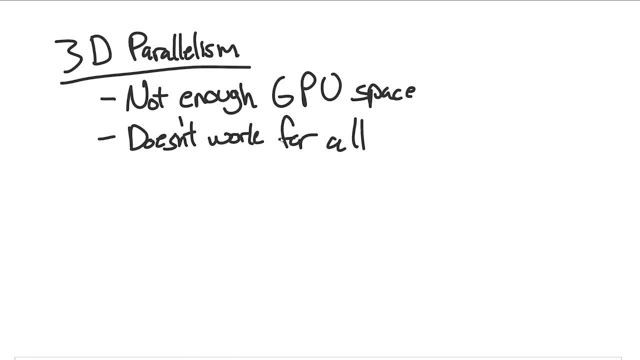 work for all models for all models that that's a huge downside right we want to be able to fit essentially whatever model in you know if we want to do super wide models we don't want to be limited 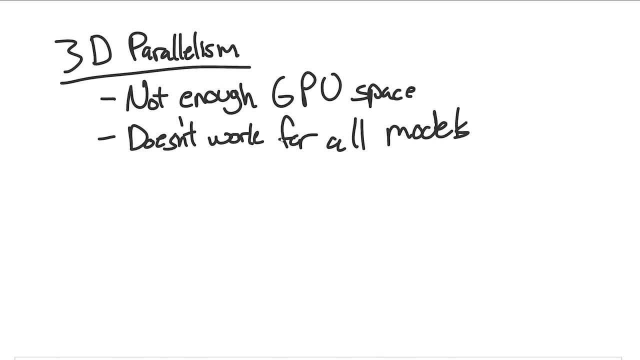 to that if we're going to be able to fit a single model then we don't want to be able to fit a single model by that. And then the other sort of downside here is that this just takes time. It takes time. It's 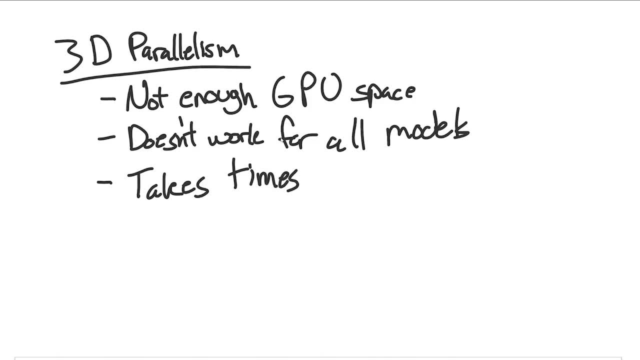 sort of a pain. You have to refactor your model to use 3D parallelism where ideally this whole process should happen automatically. You don't want to waste your time doing all this engineering 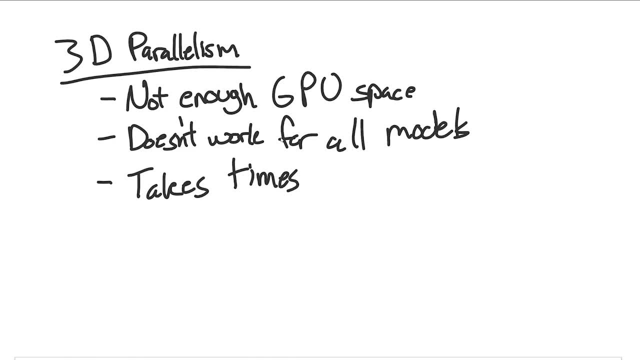 when really you just want to be working on experimenting with new ideas and seeing what works. So really the goal here is going to be, the biggest goal is to be doing this automatically. 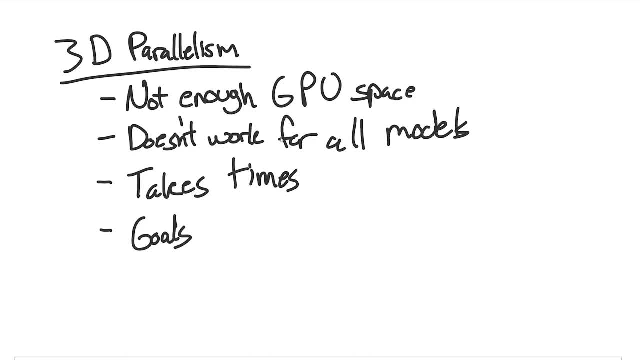 So I guess we should say goals. And this is sort of what the paper does is doing this automatically and not just automatically, but doing the scaling to not just GPUs, but also looking at CPU memory and other memory. Specifically what they end up using in the paper is NVMe, which you can think 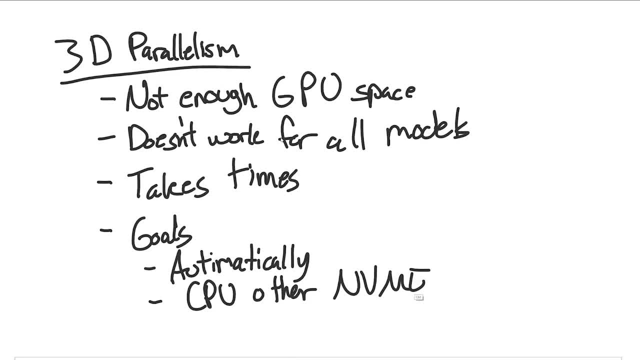 of this as, I'm pretty sure this is just SSD and the E is supposed to be lowercase if it really matters. But this is basically just SSD. I think NVMe is a way to, 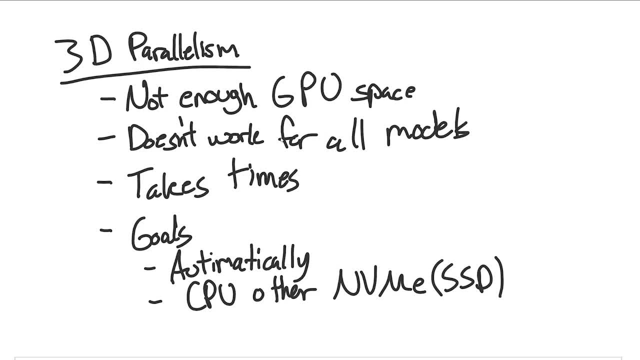 communicate with SSDs. I think you can double check that, but essentially we want to use non-GPU memory. So that's sort of the goal of this paper, just to give you a little background. 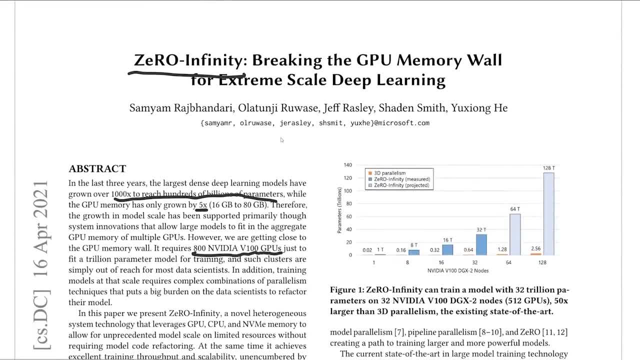 So this paper came out just roughly two months ago from now, I think it was in April and it was released by Microsoft. Unsurprisingly, the company that's not working with OpenAI that is building these huge, huge models, right? So maybe a little bit of why there. 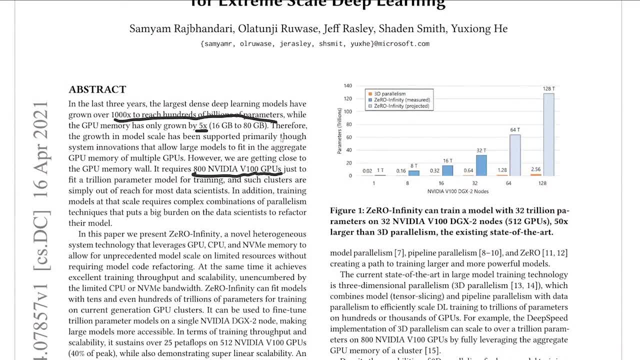 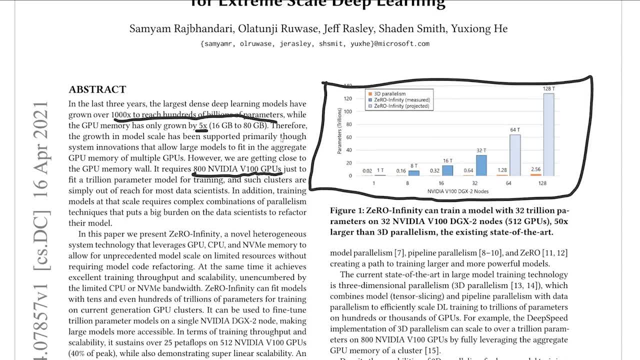 graph shows is really kind of crazy. If you look at this, this is the different scaling between 3D parallelism, which is what we just talked about in the new method, zero infinity. So they start off with NVIDIA V100 DGX two nodes. So each one of these nodes, by the way, I think has 16 different GPUs. So keep that in mind. So we can multiply each of these numbers by 16 to get the number of 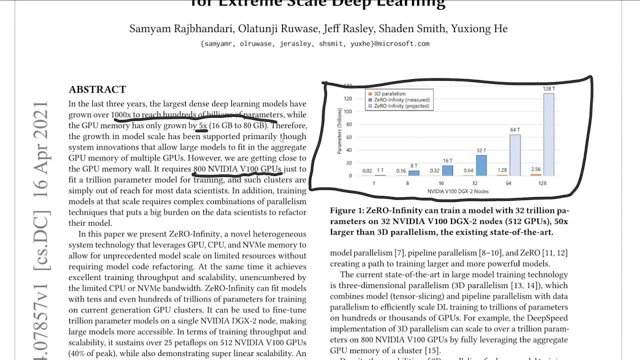 GPUs. So for 16 GPUs, they can run a 1 trillion parameter model with this new method. In comparison, previously, they couldn't even do, uh, what, what is this? This was like 20 million. No, no, no, no. 20 billion, I think. Yeah. 20 billion. So that's a huge increase from 20 billion to 1 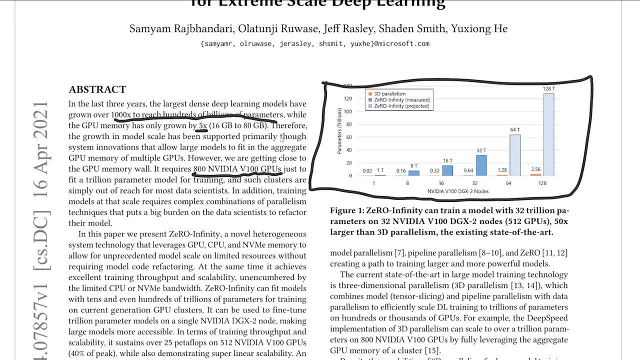 trillion. And these both scale linearly. It might not look like it because of the axes, but these both do scale linearly, which is really great. That means every time you add a, a new GPU, 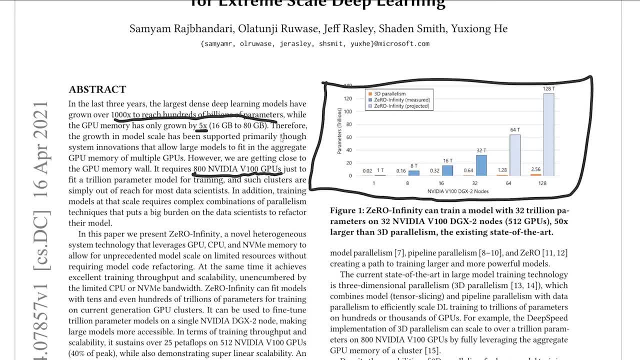 you're essentially getting an extra 60 billion parameters, roughly that you can, that you can add to your model. And I know I just said this, but I want to iterate, reiterate this just because of how incredible it is. This is 50 times better than what we had before. So if we could train a 1 trillion parameter model before with our, with our hardware, now we can train a 50 trillion parameter model, huge difference there. So huge improvements. And that's really great. 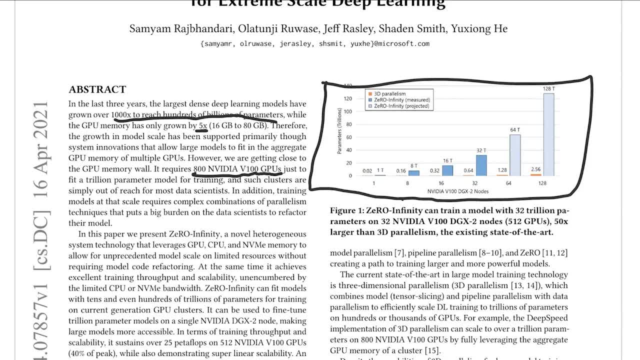 Now I will say a little caveat. This is linearly scaling, so from like one GPU, the scaling starts with 16 GPUs. So I don't think it actually starts from one GPU. It might start from around eight or something. I'm not exactly sure they don't go into that. So you won't get this as good as results. If you're using a single GPU at home, you probably won't be able to train a 60 billion parameter model. But what I found, I looked around a bit and I found that 13 billion was roughly where it starts with one GPU, which is still really crazy. That's still enough to train GPT two, at least memory wise, not compute wise, but memory wise, you could put GPT two on a single GPU. 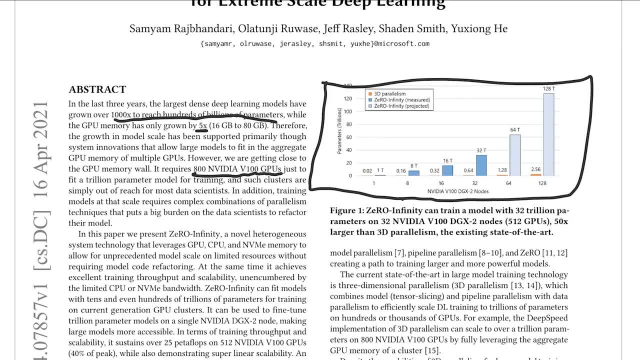 With that. So really, really great there. So that's a preview of the results, but now let's talk about how this actually works and what we need to do to get this to work. So if we actually scroll down quite a bit here, oops, they have a, sorry, my mouse is in the wrong place. They have 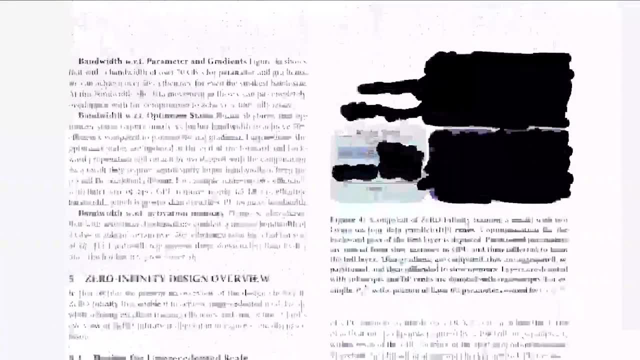 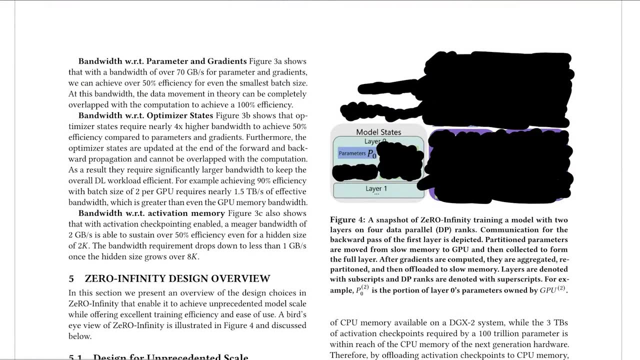 a little graphic right here that is very helpful in understanding how this works. So what our goal is essentially to take all these parameters we have and move them throughout the GPU, the CPU and our SSD as necessary, right? So let's first think about 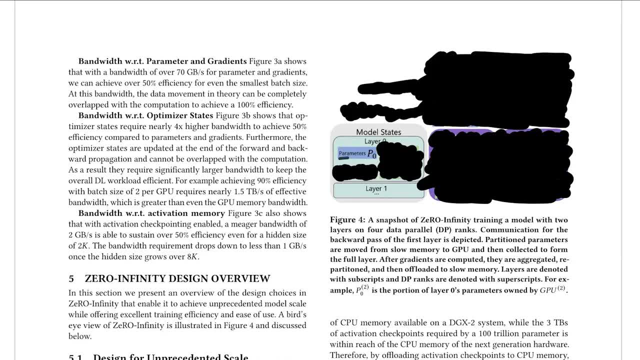 what we actually need to be storing and transferring. Well, the first thing are the parameters, right? We can see that right here. So the parameters are one thing, but there are actually two other things that take up a lot of memory. The first one you might've thought of is the gradients. So the gradients are really important when we're doing back prop. We need to make 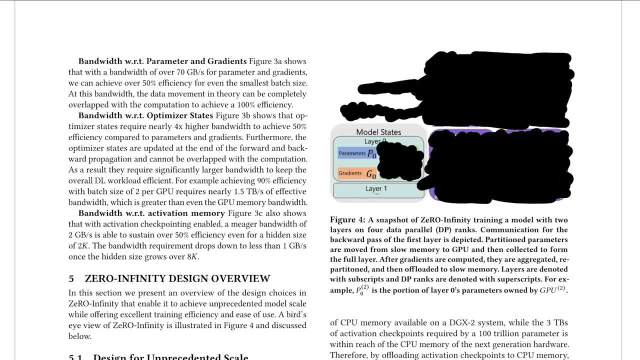 sure we have a place to store those and are roughly the same size as the parameters. What's the last thing though? There's actually a huge box here. You can see I covered up this probably you don't think about as much, but we actually have optimizer states. So this is if you're using something like an atom optimizer, Okay. 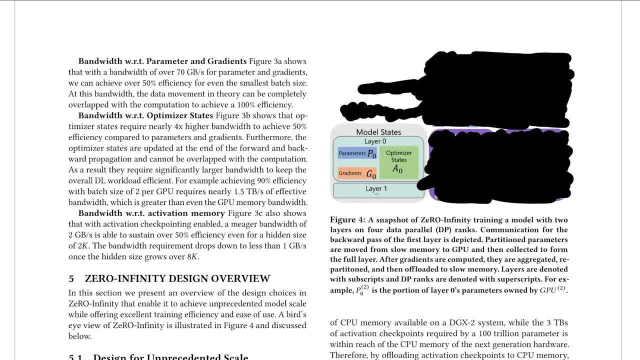 That actually stores a bunch of variables for all of your parameters. And this is very essential for training huge models, which is what this paper is all about. So we can't like throw these out, right? We need these two. So these are the three different, we call them model states that we need to be accounting for. 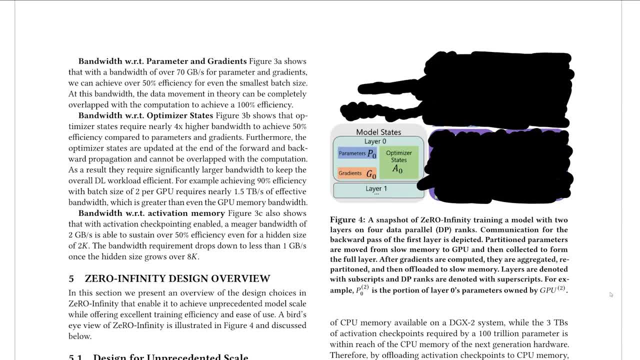 So at the very startup of this model, when you start running the training, the first thing that happens is we use the infinity or this paper uses what's called the infinity offload engine, which is something that Microsoft has developed. 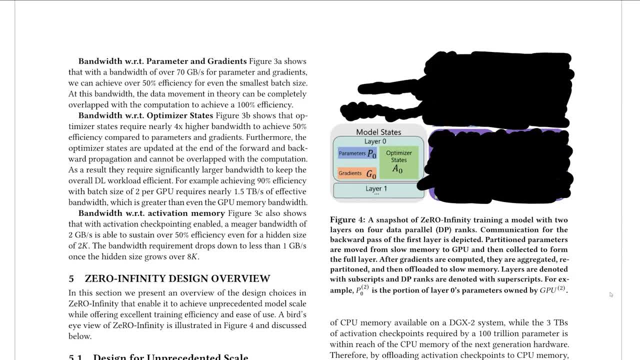 To do that, that whole thing automatically, right? We take all these and we decide what's going on the GPU, what's going on the CPU and what's going on the SSD or the NVMe. So right here, you can see. 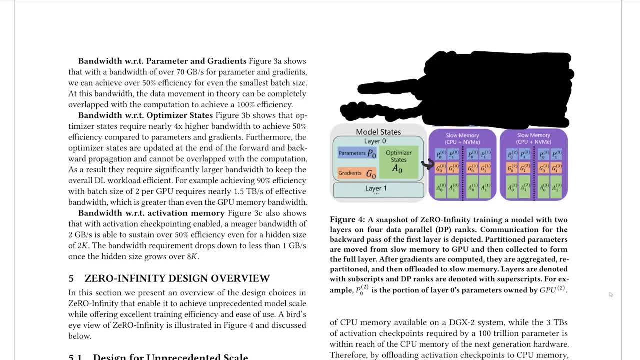 We go from here, the model to distributing this on the slow memory. And sometimes also on the GPU, if we have enough memory on the GPU. And that's again, the really nice thing here is that automatically does this whole thing. So if you have enough memory on the GPU, it will do that for you, but if you don't, it will figure out where it needs to put the 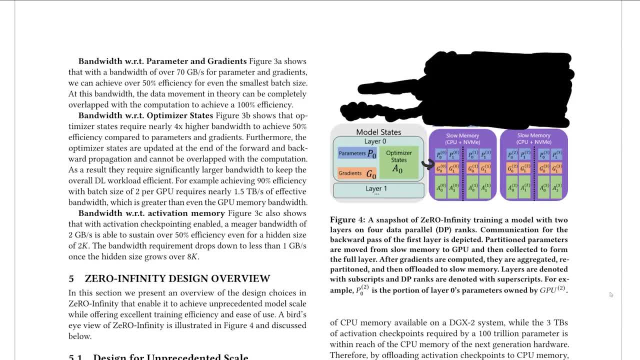 all this work out and this is sort of what we talked about earlier because the previous method 3d parallelism you had to do all this yourself well it didn't even put these here right but everything you did do had to be done manually here it's all done for you and the software is actually open and available i'll be talking about that at the end of the video so it's not like you 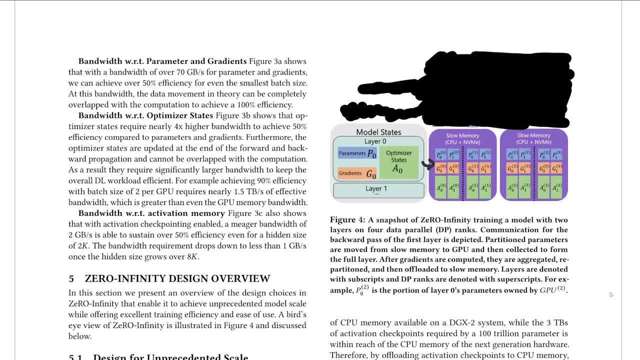 have to cut any of this very nice now the next thing that happens is we go to actually train right so we're starting to train it puts all these on the right all these parameters in the right places and now we're going to do forward step whatever it's called where we pass through all 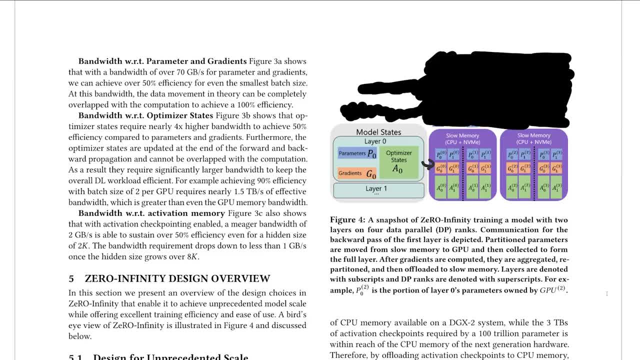 of our input data and go through layer one layer two layer three and what actually happens is most of this memory is not on the gpus so you can see here the gpus are actually reserved if if we don't have enough memory they're reserved for actual computations so when we get to layer zero we will 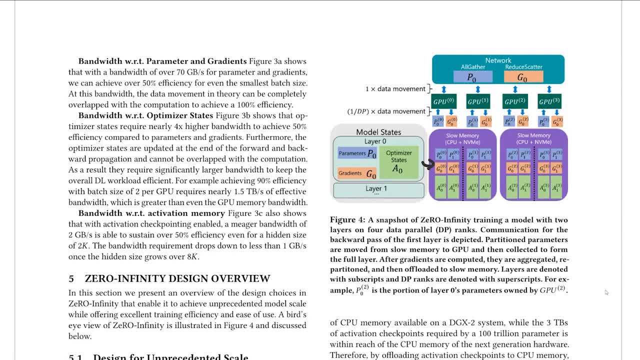 essentially say okay let's grab the parameters for layer zero pull them up into the gpus do the computation 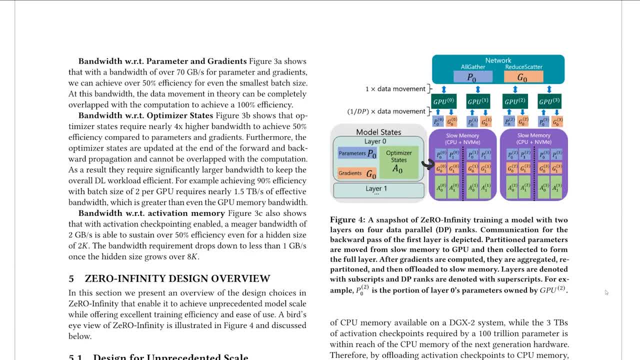 and then pass them back down and that's what you see here this all gather and reduce scatter it's where essentially the all gather is gathering all the different parameters because they might not all be on the same devices so it's gathering all the parameters from that first layer pulling them up to the gpu and then once we have calculated the gradients we can send them back down to be with 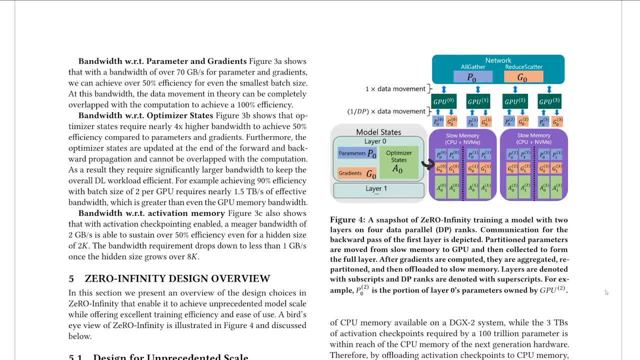 the corresponding parameters so that's that's what's happening in this little graphic here now that is all great and all so so this is pretty cool but it's nothing groundbreaking particularly because right there's 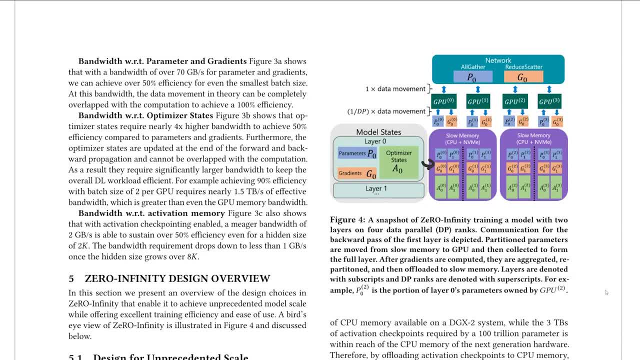 there's some cost associated with all these operations especially you know talking between the cpu and the gpu is is quite costly it takes time so you might be thinking well won't this be a bottleneck or maybe will the bandwidth be a bottleneck there's all these sort of different 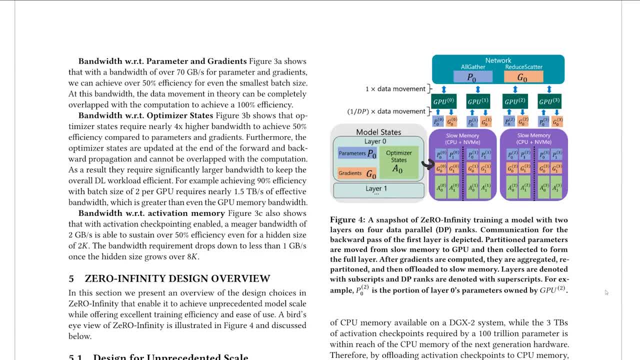 issues we can have so this design is cool but this isn't actually where the innovation comes in this is sort of the easy part what's really groundbreaking are three optimizations in particular two for speed and one that allows very very large models so let's start with that lastp on eie دیمت زوج جرامي مضل جمعجم 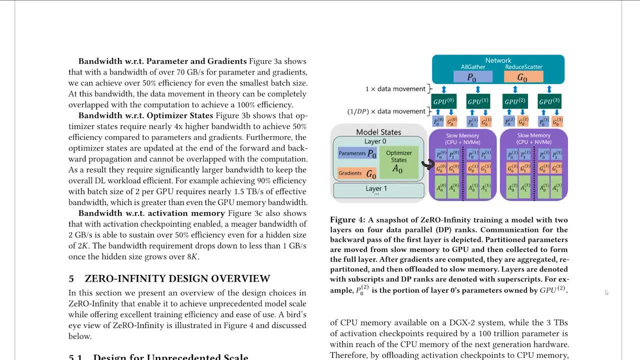 allows very very large models so let's start with that last one the one dois değil أولا أنا زوج Venice Aclam that allows for very large models and I'm going to zoom out a little bit here and sort of write 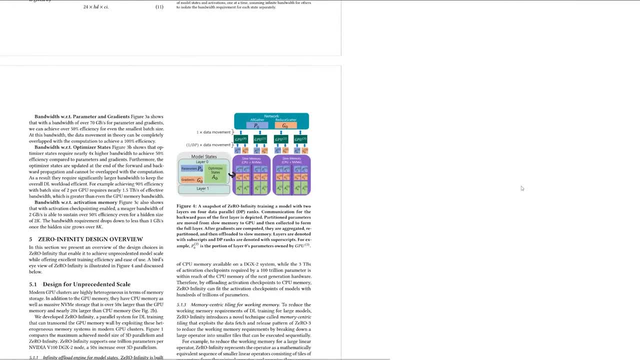 these on the right here. So the first thing is the memory centric and they love this word centric. I 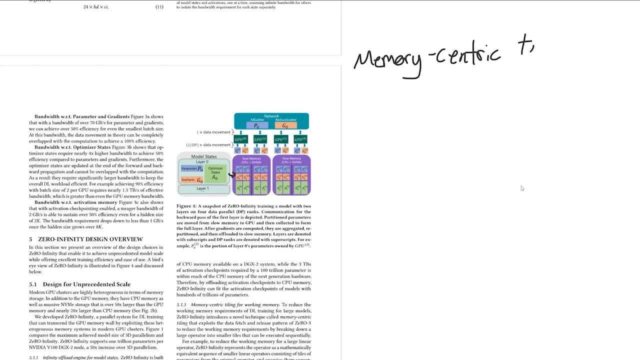 swear they use it a trillion times in this paper. Memory centric tiling and essentially what memory centric tiling does is it breaks up singular layers. So sometimes we don't have to do this 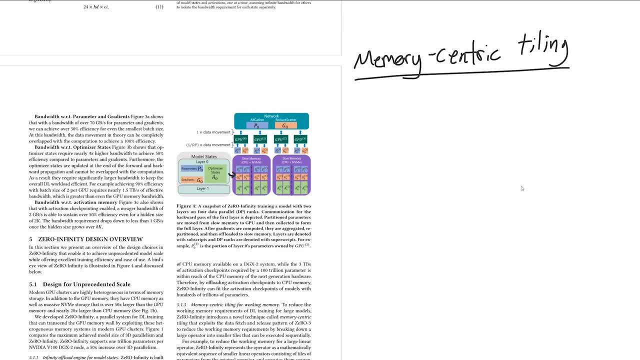 but occasionally we will have models that are so big and so wide that their single layers can't 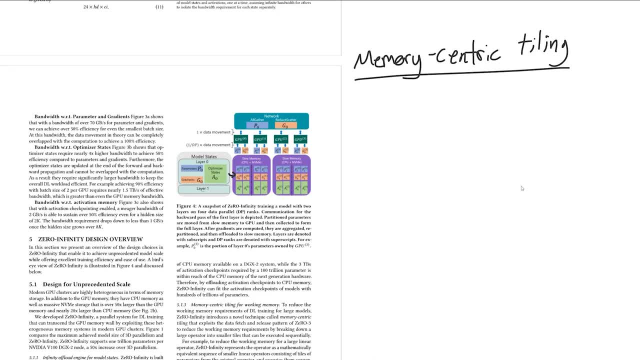 fit into GPUs. Remember this was a drawback with 3D parallelism. At that point in if we were using 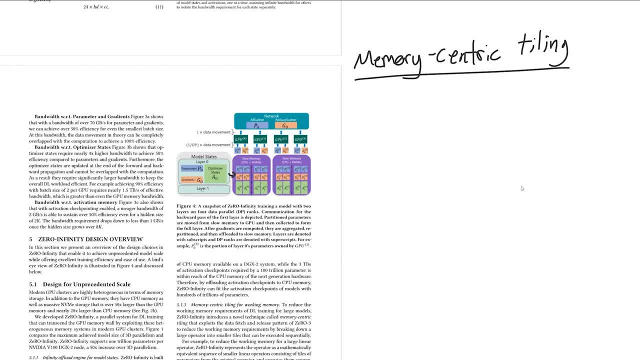 the previous model well there's just nothing or the previous method there's nothing we can do here 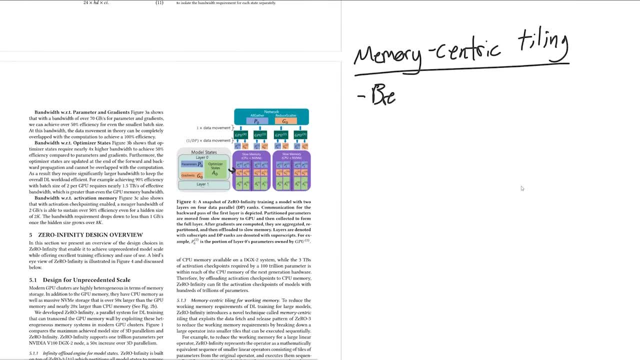 but here what this actually does is it breaks up layers. So it breaks up layers and stores their 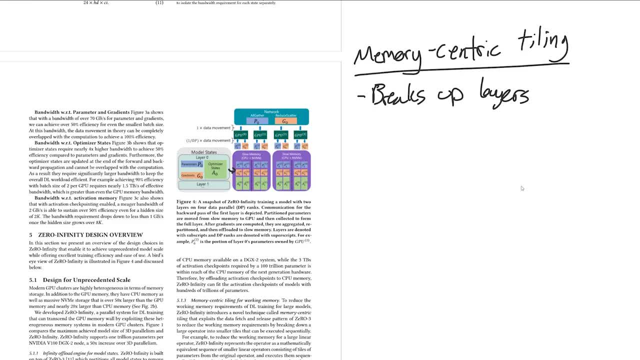 parameters in different places and then pulls them together separately and performs the calculation 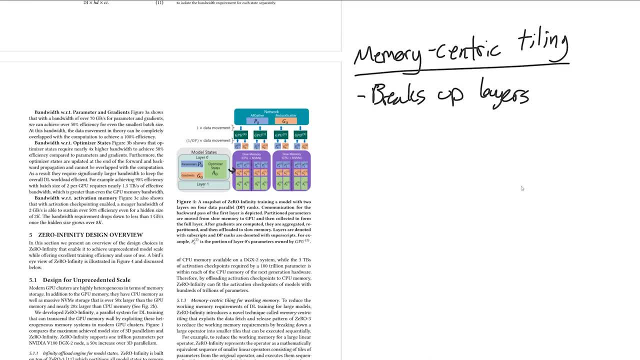 separately. This means that no matter how big a layer is we can still break it up and we don't have to worry about running out of GPU memory. 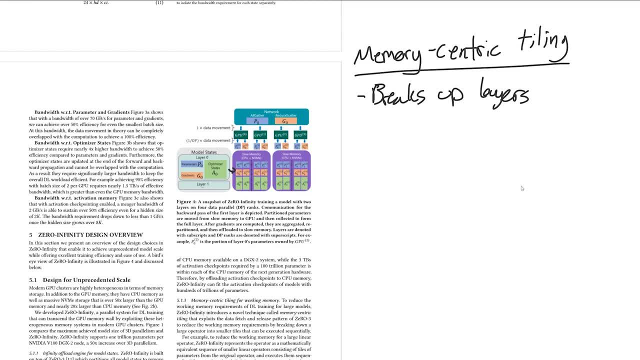 So this is a great way to essentially increase the width of models that we can compute. So that's optimization number one. Optimization number two is bandwidth. Bandwidth 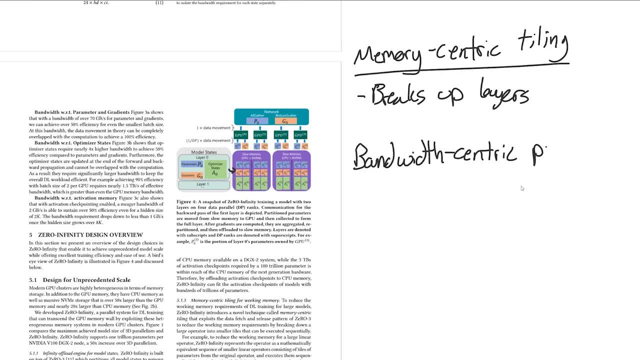 centric. Again centric you'll see this a lot more. Partitioning. Now to be honest this is uh there really isn't too much interesting stuff about this one. This is probably the most boring of them all. But all it is is it's saying the 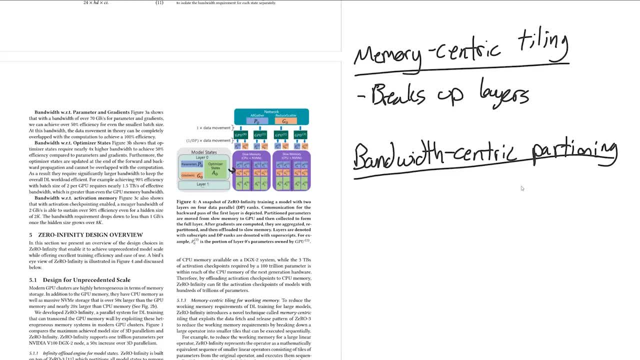 the bandwidth that we use communicating between the CPU and the GPU we need to make that you know we can't have that be constant we need it to scale every time we get a GPU because if we don't well 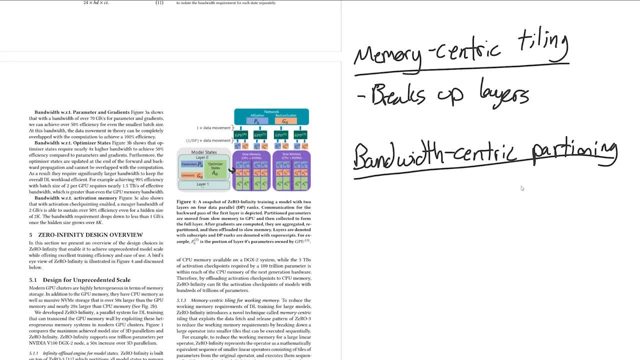 we're going to run out of bandwidth right this is supposed to support many GPUs. And essentially what they point out in the paper is the the specific way they do the message passing and the parallel computing here using this all gather method as opposed to like there's other ways you could do 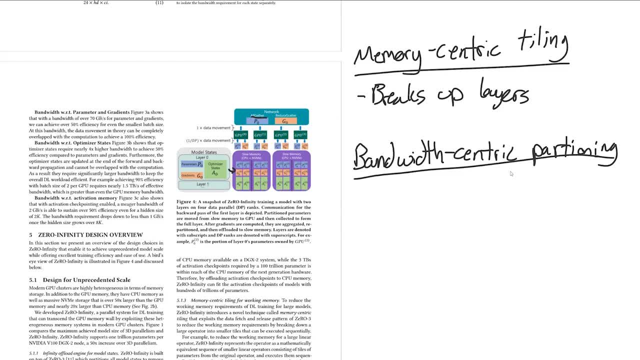 this using like a broadcast method if you don't know what that is no worries all that you need to know is this all gather method specifically that they use makes this linearly scaling linearly 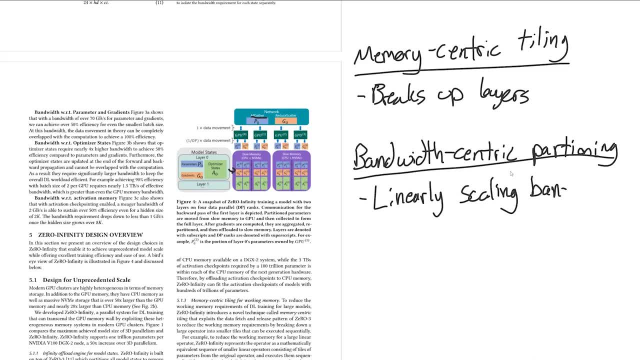 scaling bandwidth which is great that means every single time we add a gpu so if we have five gpus and we add five more that means we're now getting double the bandwidth which which is great now that 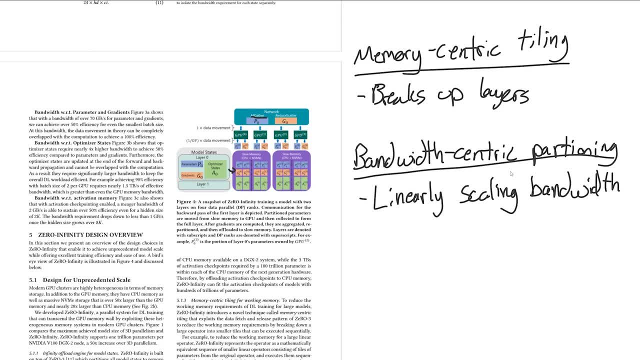 doesn't mean this can't still be a bottleneck right bandwidth even if we are linearly scaling 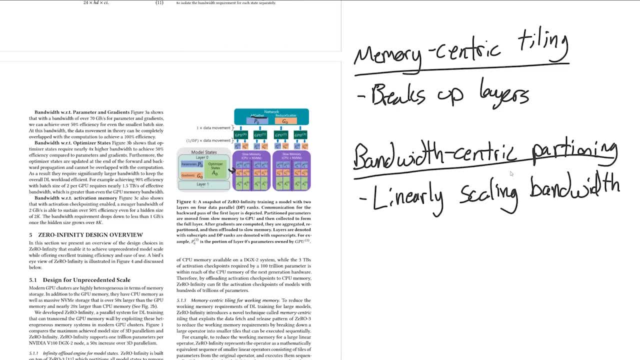 maybe that isn't good enough and that is where this next sort of optimization comes in super handy and that is overlap centric design i'm actually going to erase these two sorry but this next one is very important and it's going to take up a bit of space i think so let me erase these for the most important one and this is where i think this really is is really interesting 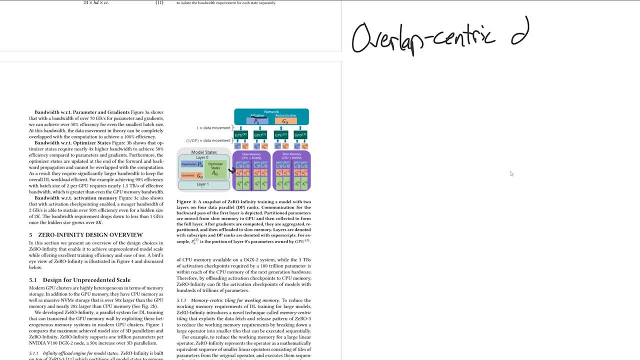 centric design design i can't spell right now uh there's the centric again they love that word i don't 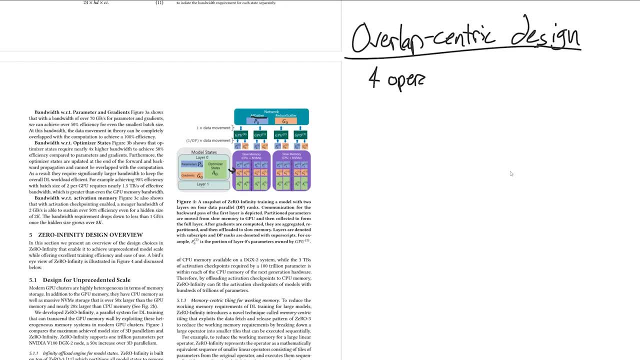 doing this whole thing right so four types of four operations the first one is we need to read from cpu right so we might need to read the parameters from the cpu we then need to copy to gpu right so we need to talk between the cpu and the gpu and this by the way usually takes a long time if you've ever trained lots of models you know you shouldn't be doing this all the time uh so so you know this could certainly be a limiting factor even if we do have linearly scaling bandwidth but we're going to talk about how they get over that in one second so the next piece is they've they've gotten all this data on the gpu now they need to gather it 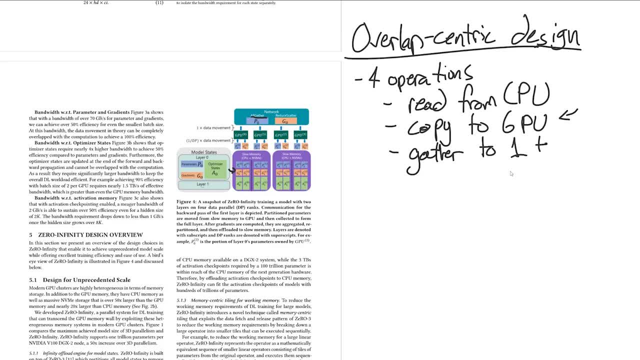 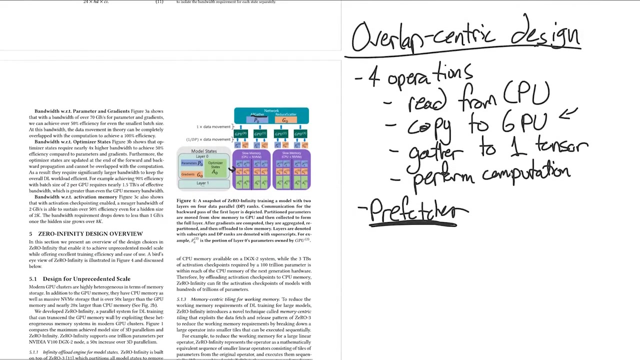 up in a VeryPusher template to play around with them right they do all this하고 in doмер and then the fifth study says right so this is similar to when we do a load for hundreds of std or tns you have the two same things there that are going to be thrown in call right because that's what we need you know because we need to collect them and we need to get from the environment doing one after the other we could very easily run into an issue of not doing this fast enough so the whole idea is that we want to do all these operations in parallel and the way it does that is with a prefetcher because and i'll i guess i'll prefetcher write this out first this is the key here this prefetcher now we can't copy something from the to from the cpu to the gpu if we haven't read it off the cpu yet we can't gather things into a tensor if we don't know what those elements are yet and we can't perform a computation if we don't have a tensor to do the computation with yet so how do we do this in parallel and the answer is that we look many many steps ahead and start calculating steps ahead before we even get here so the prefetcher at runtime which i think is really cool it does this at runtime you don't need to define well i guess you do sort of have a graph defined but not in a super complicated way like you used to in tensorflow or anything but the prefetcher will look ahead right it will look ahead 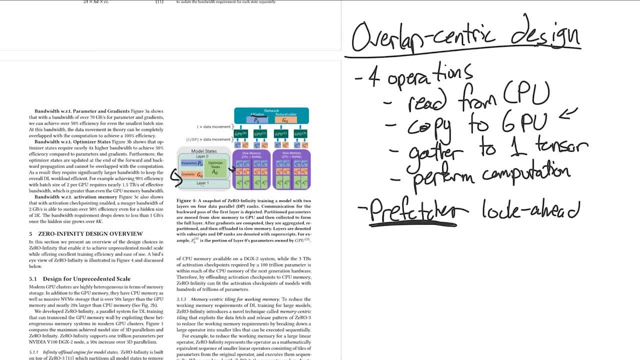 at the layers to come so say we're on layer zero it will look at layer one and it will say what are we going to need well we're going to need parameters uh p1 or and or whatever parameters 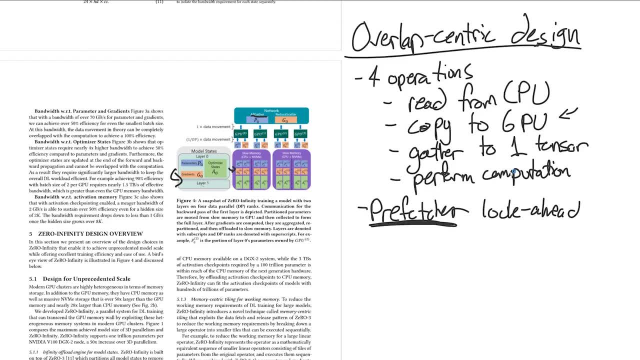 there are and it's going to start these steps already and if it has more bandwidth it might even jump ahead to the next layer and start the steps even while we're still doing the 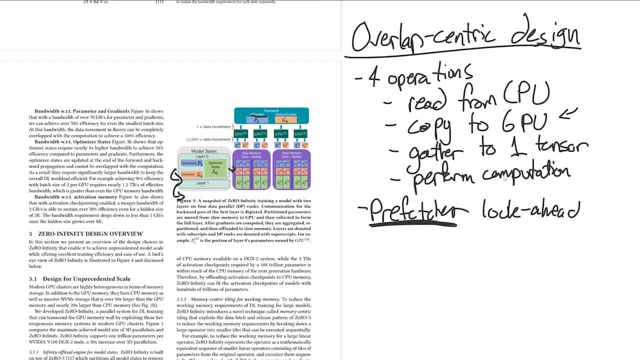 calculations for layer zero so it will start doing all this so that by the time we get to that layer we already have our tensor and we can start the computation 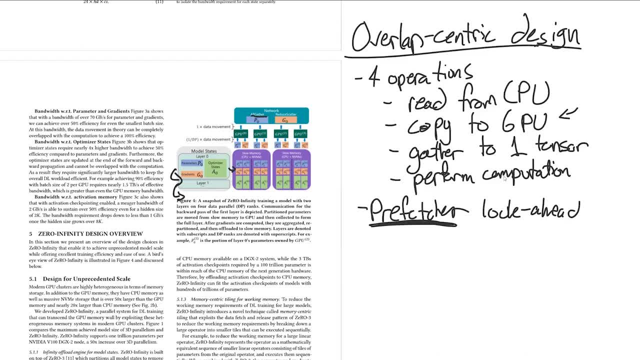 that is the way it essentially it's it's really really aggressive parallelism which is incredibly cool and this is where the systems design really comes in if you've ever learned about how computer 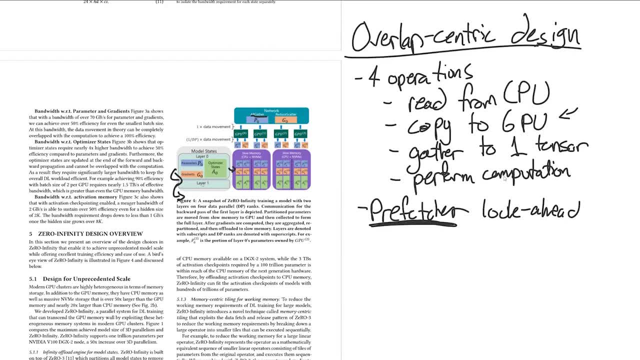 computations work how like the clock works and how you overlap essentially all these different operations this is probably going to look really familiar to you and it's really neat that they're 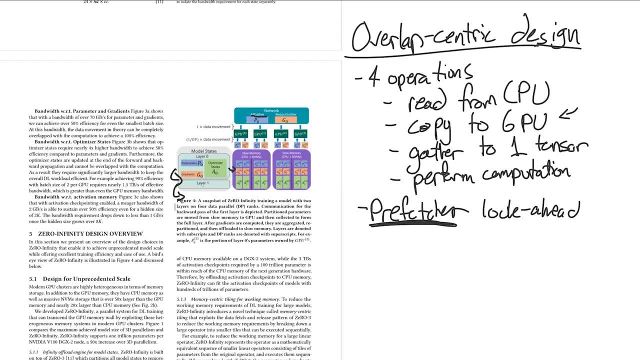 sort of bringing this into ml this super efficient design that we built out for computers you know many years ago and that's why that's the one of the reasons i really love this it's really just 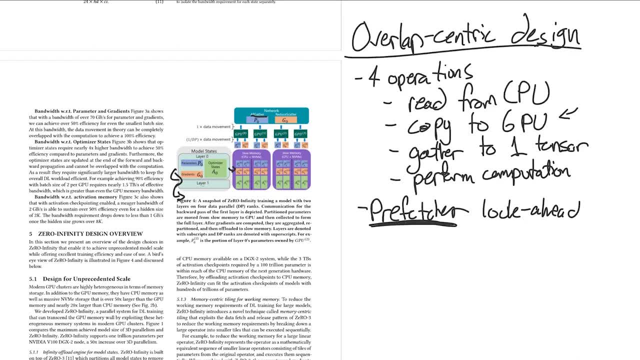 been optimized to the core super super efficient parallel computing it's cool you know you can't get 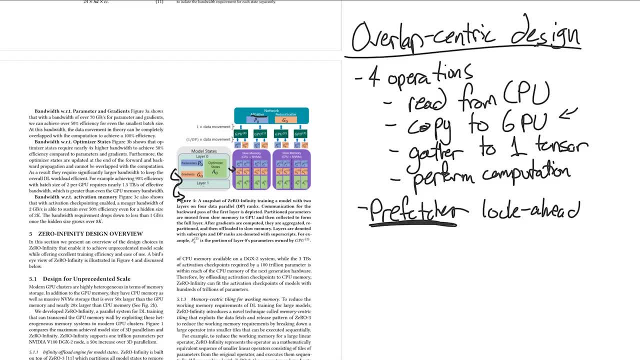 around it it's cool stuff so this is especially really good for a low gpu count uh low gpu count so this is you know uh if you only have two three gpus or even one this is going to be really great 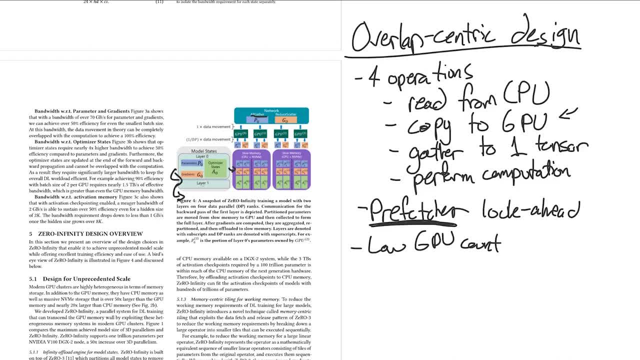 because it's a lot harder to do this uh when you only have it's a lot harder to be fast generally when you have one gpu and you can't do these parallel computations as much but if we're doing 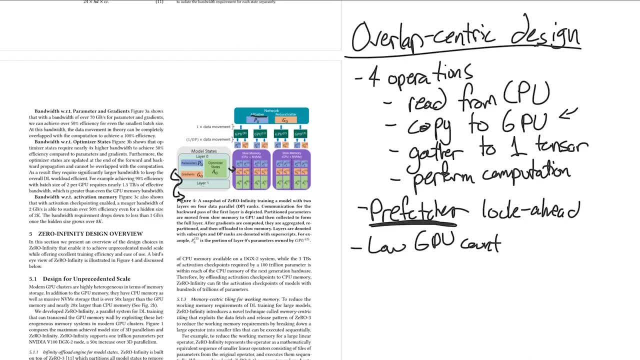 a lot of these parallel computations we're going to be able to do a lot of these parallel computations and this ends up helping us out a lot more so this is really awesome and the end result is just crazy efficient parallelism that's sort of an overview of how this whole system works pretty 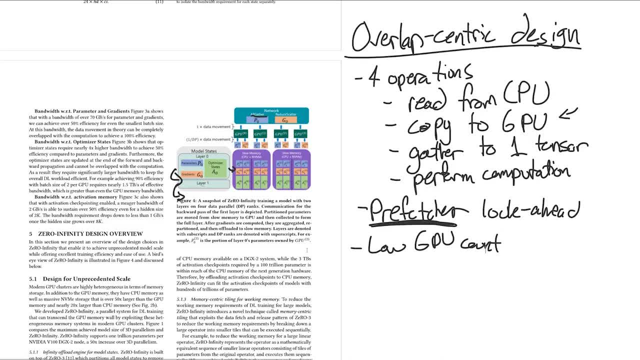 neat right and you can read through the paper if you want more details the paper or the paper here mostly details for the math how they came to these numbers and stuff it is interesting but this 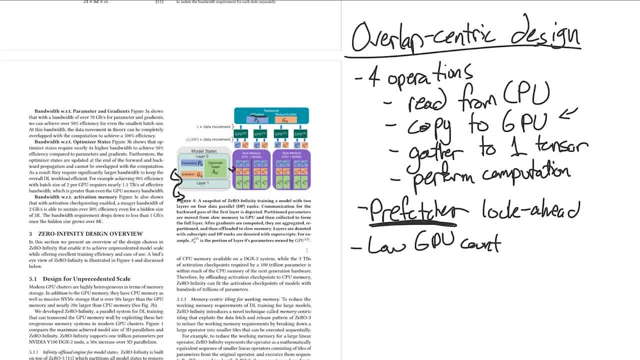 hopefully this gives you the general idea so your next question you might be wondering about is what about the results what do the results look like 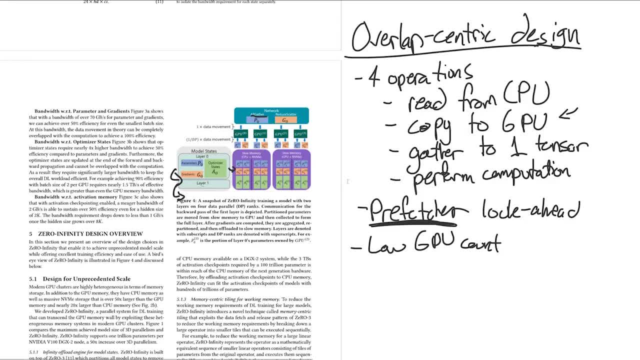 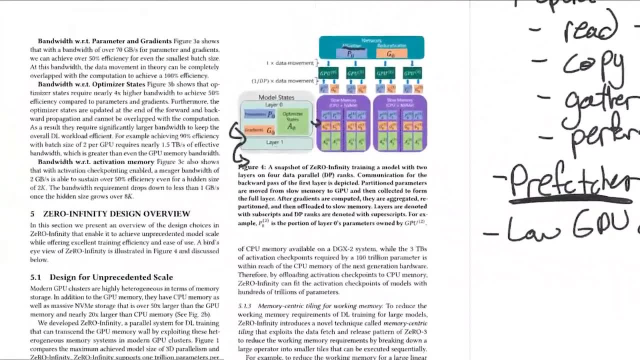 and that is a good thing to question so let's go ahead and take a look they have a few graphs down here let's zoom zoom back in uh oh no oh no uh uh there we go so if we zoom down here we should be 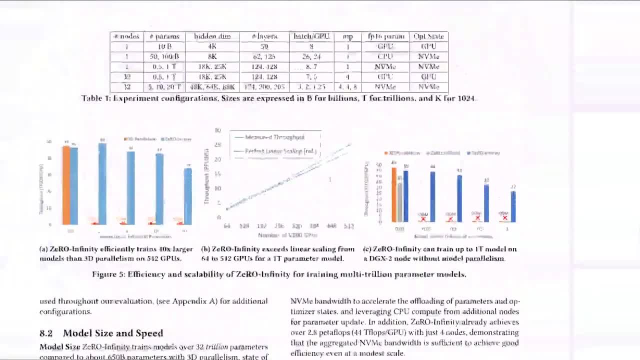 able to find a few graphs where are they where are they long paper here we are here we are so here they compare the throughput now the throughput you can think of essentially as the compute how 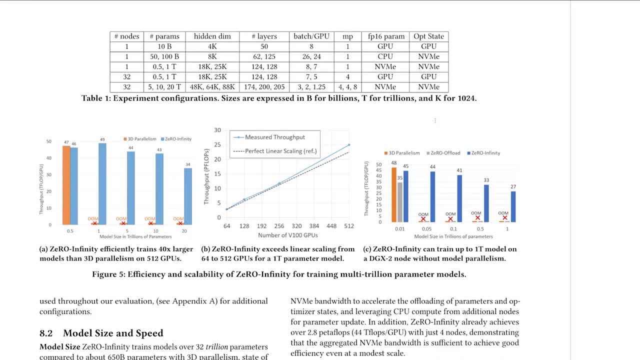 much compute we're getting how fast things are running that's probably the simplest way to put it so the higher the throughput the faster we're training the model even if we can fit these giant 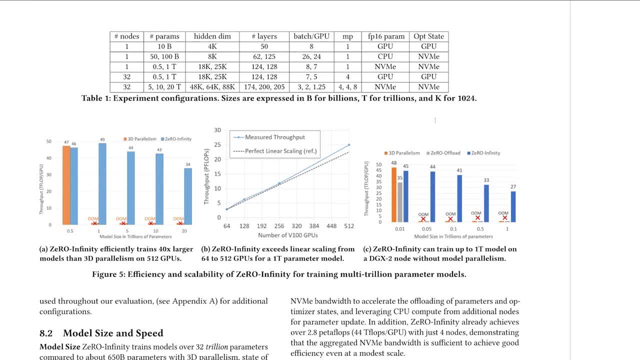 models onto a small amount of gpus we still have to compute fast enough to train them so that it doesn't take us a trillion years right that's pretty important so looking at these the results 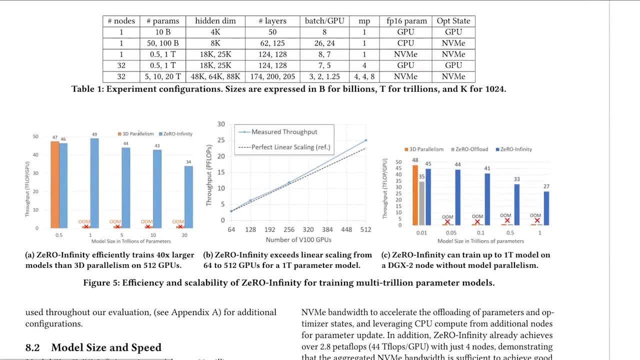 are actually pretty good now you will see that they don't actually have comparisons with 3d parallelism for lots of this because they didn't have enough resources because it goes um so fast 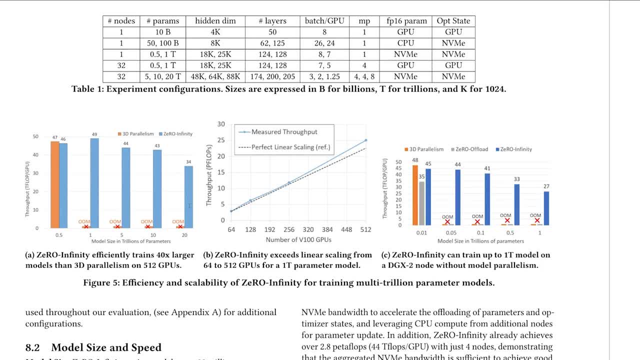 you really can't blame them it would have cost them millions of dollars probably to run these tests 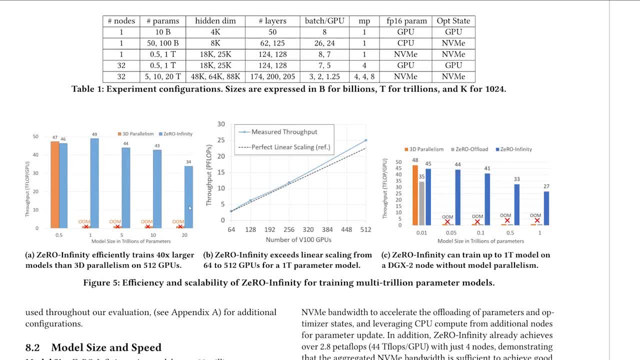 so you know um yeah um well i say millions i'm just pulling that number a little bit out of my butt uh i just looking at gpd3 though they might have not had as many epochs and such anyway it would 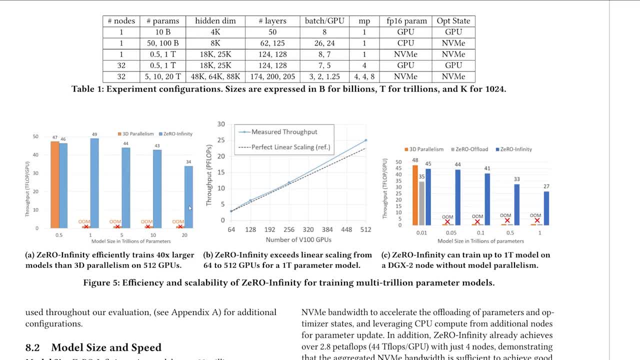 have taken a lot of money and a lot of resources that's why they don't have the comparison so just thought i'd mention that but if we look so the first thing they have is throughput with the 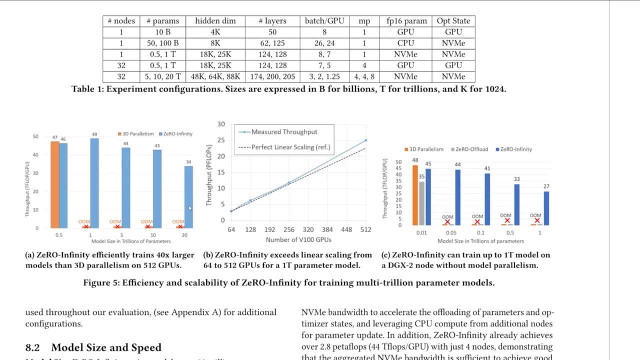 model size on 512 gpus keeping that constant and you can see this does decrease a little bit now it does increase at first from 0.5 trillion parameters to 1 trillion parameters and that's probably 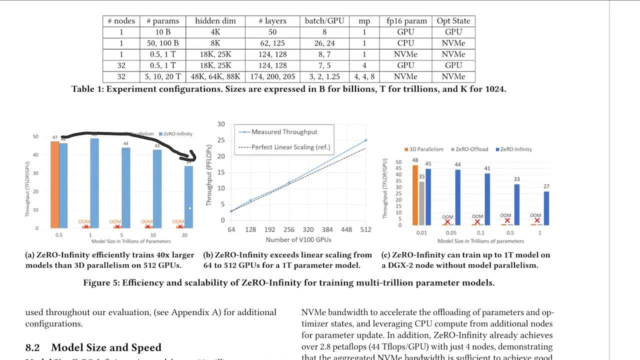 is it's not perfect but it's pretty good it's pretty good and it doesn't drop that much at all you get to 10 over 10 trillion parameters and i mean we're we're still working our way towards 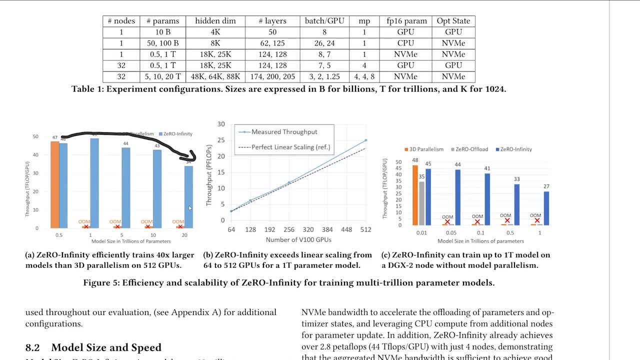 10 trillion parameters so i give this a seal of approval for me at least the next graph they have right here is the graph on uh throughput with the number of gpus and what is actually i found this slightly surprising i guess maybe not because again this goes hand in hand with parallelism 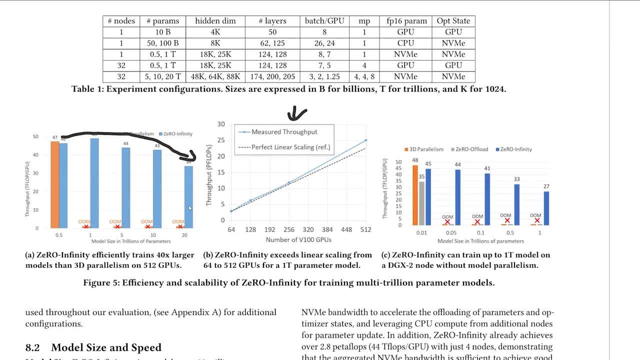 is that the more devices you have to work with the more efficient you are but what's really crazy is above linear scaling now it's not super above linear but it is slightly above linear which 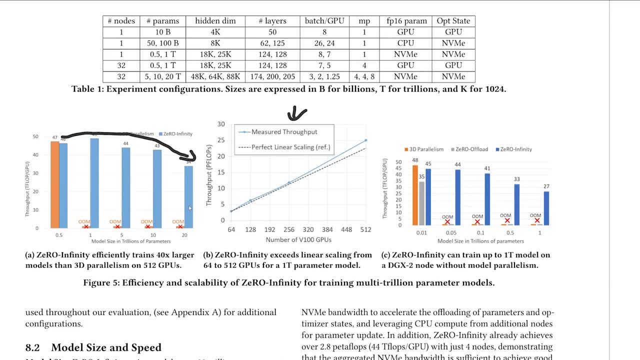 means that if you go from 64 to 128 gpus and then from you you double that again from 128 gpus 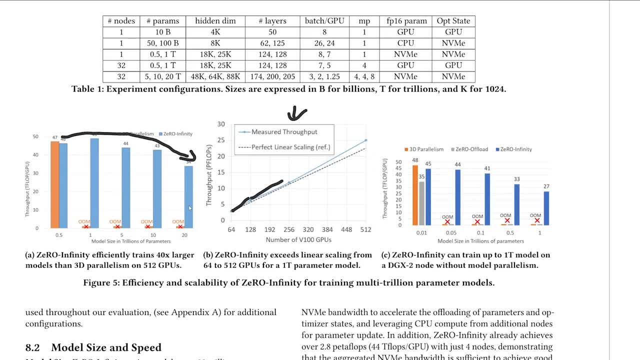 to 256 gpus well you don't just get you know let's say you get x improvement from 64 to 128 and then you go from 128 to all right i should say 128 to uh what's 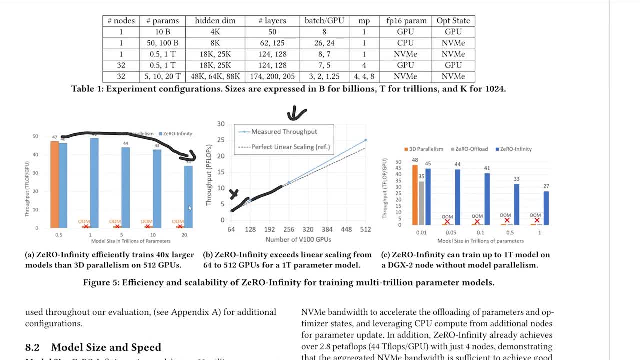 that plus 64 192 so this is x now this oh dang it i keep to 192 there we go so this is x now this isn't just x this is x plus some constant right essentially all i'm trying to say is that when 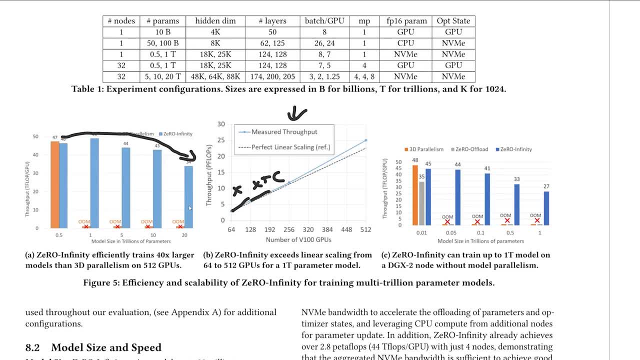 you add the same amount of gpus you're getting better returns each time which which is really great so this is this is very impressive also gets my seal of approval very much and i don't know 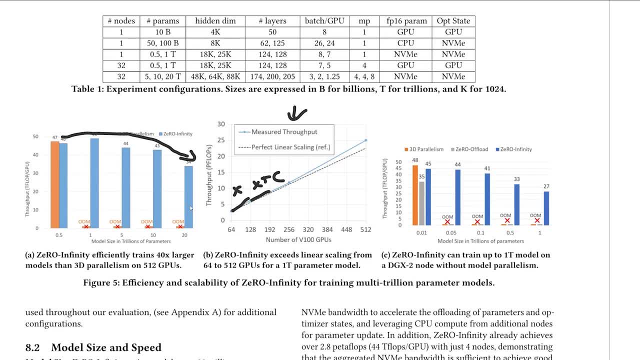 what my seal of approval is worth but um it gets it either way and lastly we can see on the right 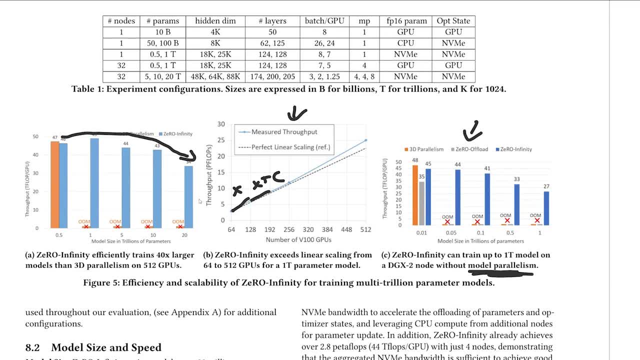 here the results without parallelism which is kind of interesting um i guess they just want to prove that the parallelism is working and if we do look we can see a huge downscaling here so there there clearly is some good work going on here this is i think where the 40 decrease was yeah this was a 40 decrease so the parallelism as i mentioned is is clearly doing good work here there's there's really no doubt about that 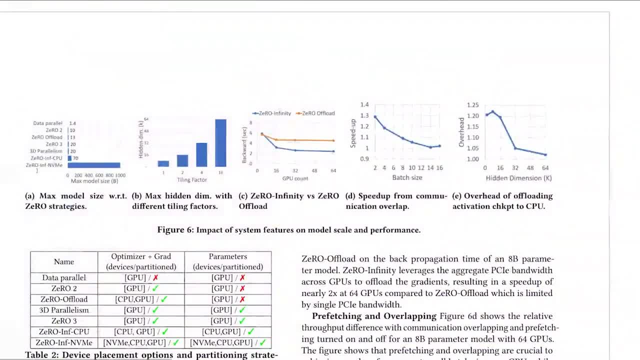 now they do have a few more results down here if you're really interested i'm not going to go through these just because i i feel like what i've already went through gives you sort of the picture of how great this is down here is a little bit more just more details so i'm going to link this 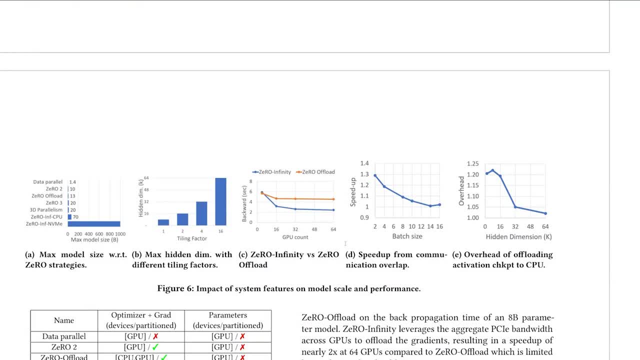 paper in the description if you do want to go through it though i do have a little bit more i want to go over though before we end the video and that is how you can start using this yourself 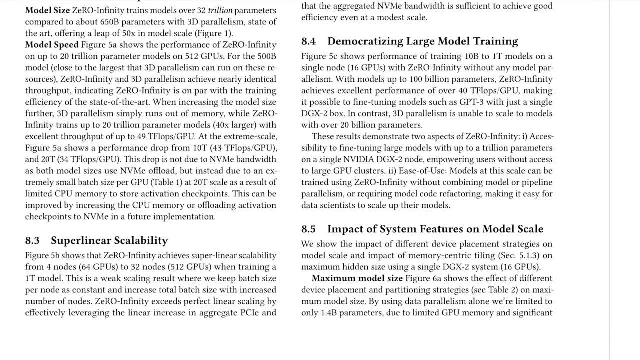 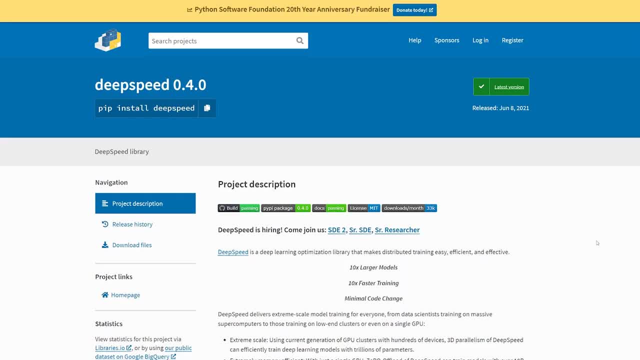 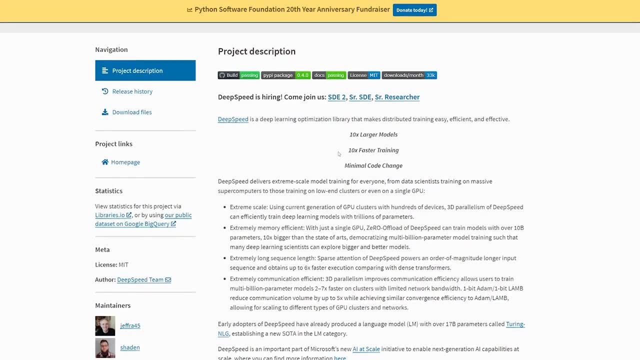 now since this paper has come out there has been a library called deep speed and i will actually pull up the page for it right now the pie pie i don't know here we go so this is the page and as you can see deep speed is a library that utilizes all these things we just talked about now it actually existed i believe before this 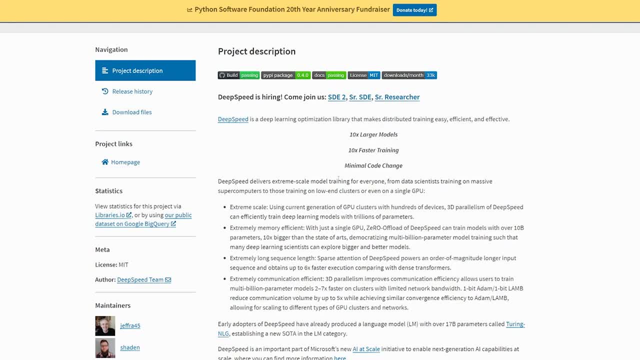 paper but it used sort of previous methods but as this new paper came out they implemented these new methods within this library so this is something you can use and they actually have 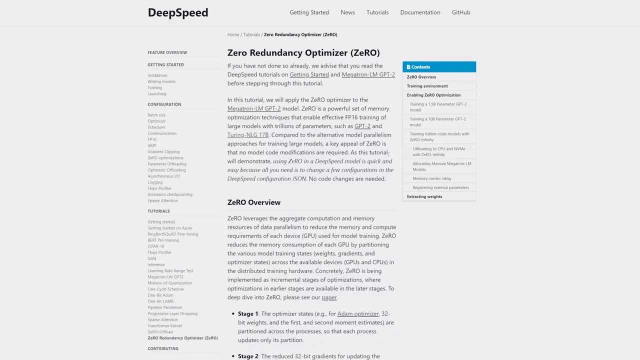 a tutorial here i'll bring this up too as to how to use this now i'm not going to go over in depth this tutorial in this video because i think that's a bit too much but what i can tell you is that 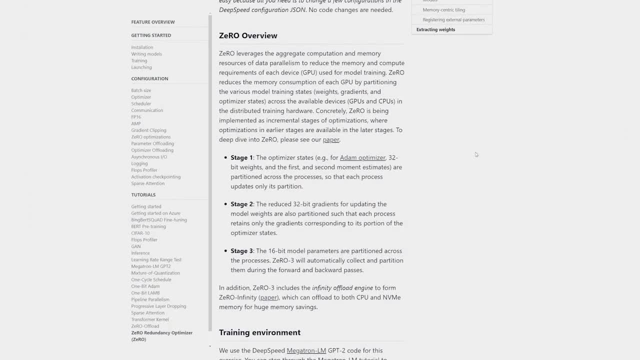 i can tell you because i've looked through it is that it's really easy it's surprisingly easy it supports everything that's on the paper and all you really need is is a config now that i guess 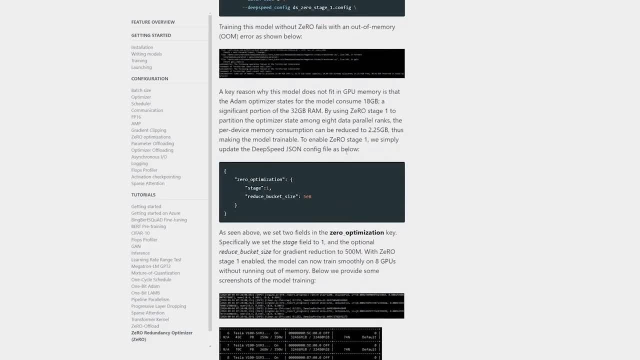 maybe there's a little bit more to it but if you really want to make this simple what i really i think goes above and beyond is that this is already implemented in popular libraries like 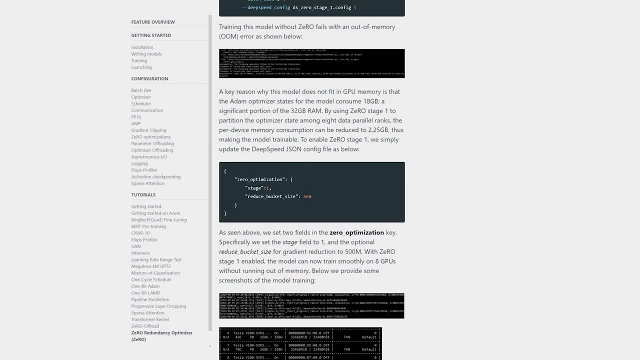 pie torch lightning and hugging face i haven't looked at the lightning implementation but i have looked at hugging face and i oh i didn't link anything maybe i'll link it in the description 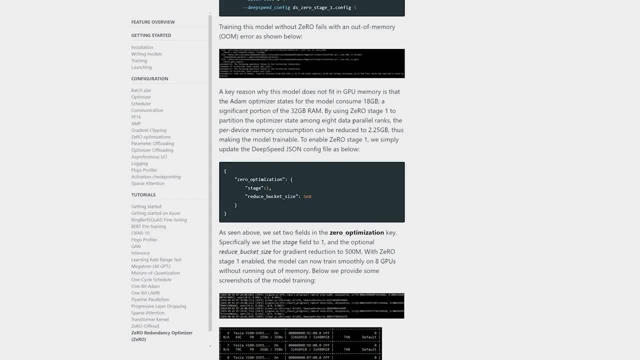 but if you do look at the implementation on hugging face they have a little tutorial all you need to do is nothing more than what you were doing before when you were doing hugging face models right it's all the same except 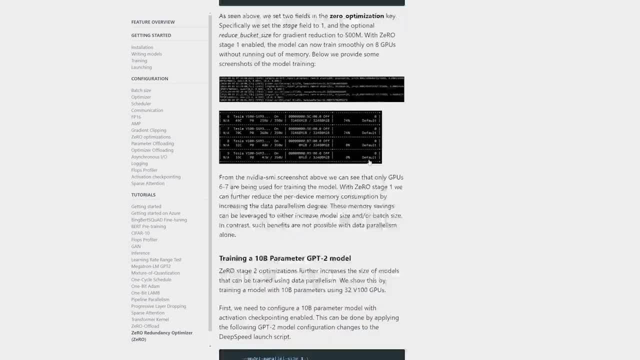 for you add one parameter that just specifies a config and the config files aren't too bad they look something something like this right it's really not too bad it talks about just how you 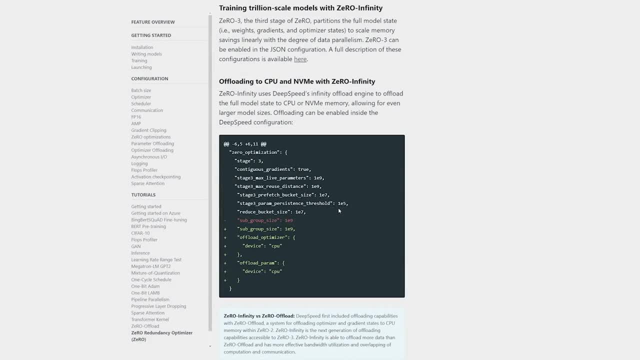 want to you know uh bucket sizes all that random stuff and they give you some presets here so it's super easy it's really great you can get onto this if you want and and make models i said earlier i 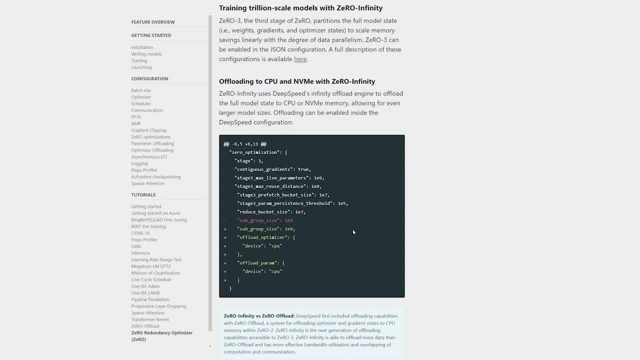 did a little digging in with a single gpu you can it depends on the gpu but you can model roughly up to 13 billion parameters is what i was finding which is insane that's gpt2 uh almost tenfold 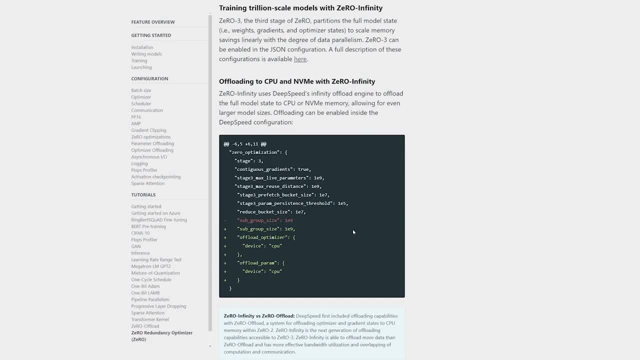 so you can you say you can definitely get gpt2 running on your own gpu as long as it's not too bad and yeah i i think this really speaks for itself it's it's a great paper 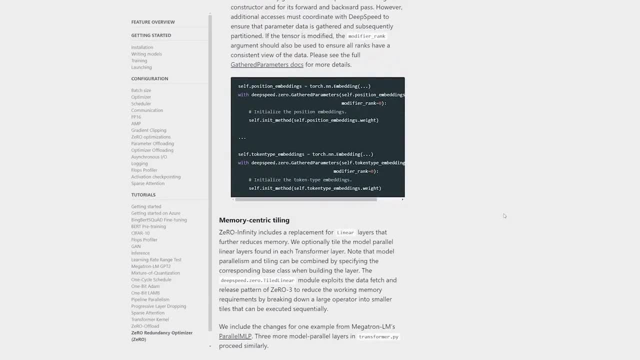 the library is already out which is super awesome and i'm really excited to see what people do with 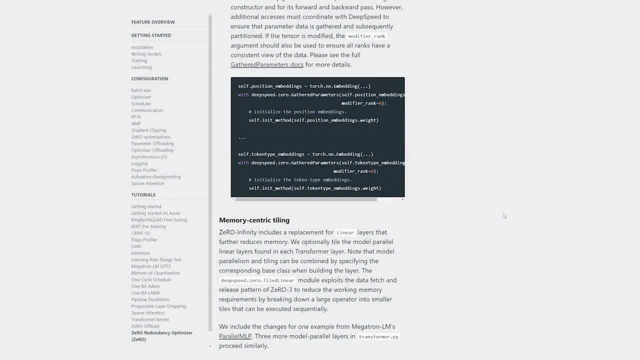 it you know i think uh openai has been one of the few companies that's been doing these super huge 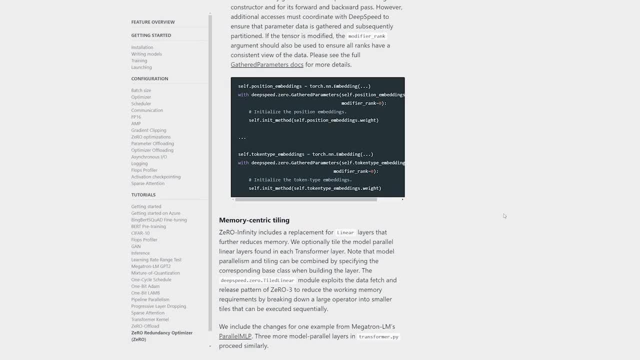 models but more recently i mean i guess google and facebook to an extent too but more recently 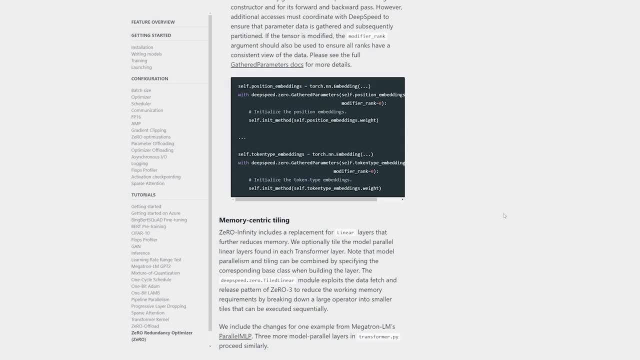 we have seen more companies coming out with these huge models i know neighbor is a i think a korean 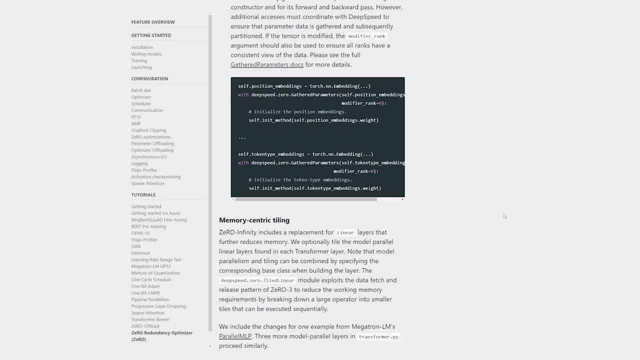 company that came out with a korean model recently i think we've seen some out of china too 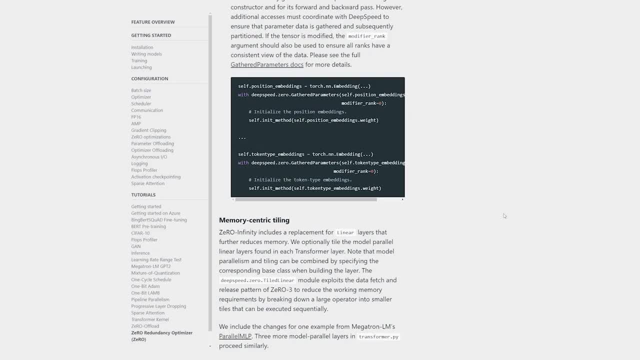 i i don't know what organizations i haven't really looked into it but you know it's really 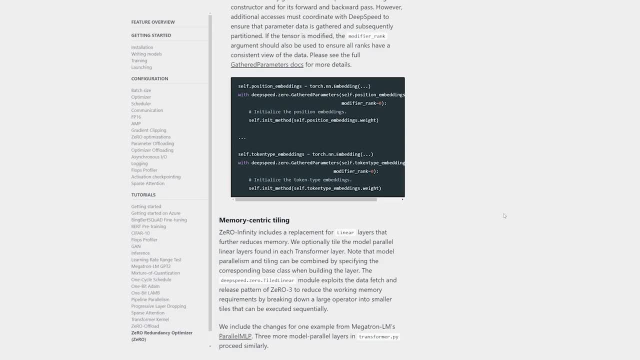 cool to see the rise of these huge models and i'm excited to see what comes from them we really 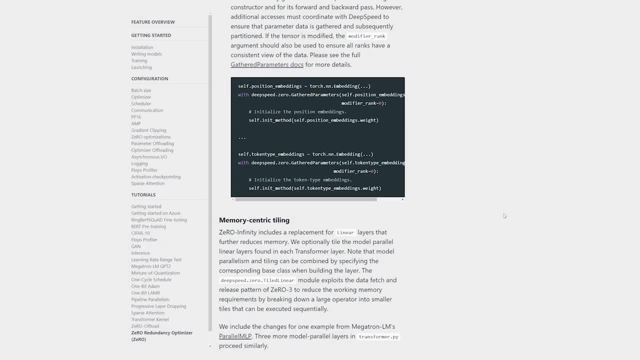 don't know and we can't know until we implement them and test them out so that's really all i have 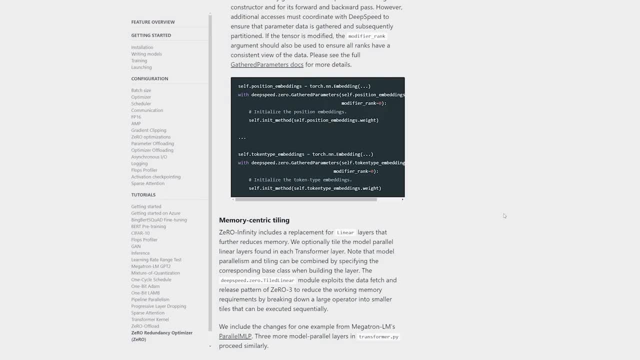 to say for this video if you like this type of content though i do a lot of talking about 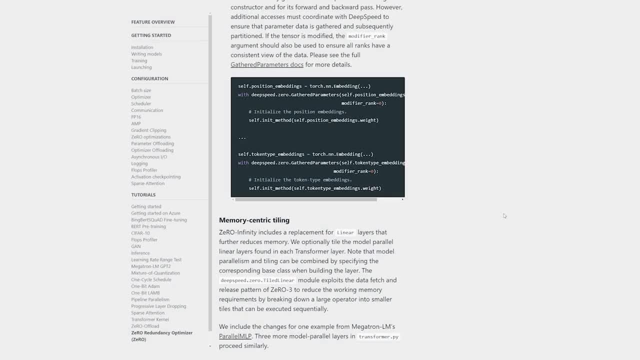 research and all this sort of thing so if it does interest you do consider subscribing it it means a lot and i'm gonna keep keep working my hardest to put out some good content but that's all i have for now so thank you so much for watching and i hope to catch you next time 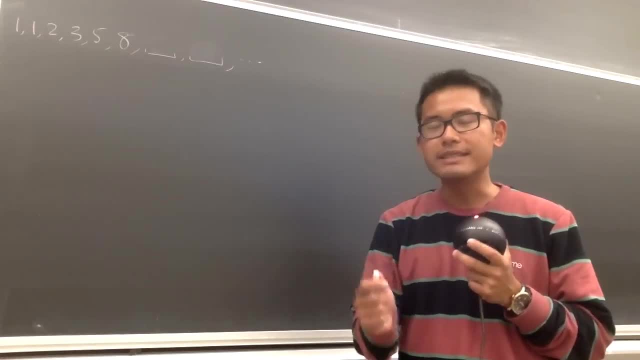 In this video I will talk about the Fibonacci sequence, and the most important thing is that I will show you guys how to find the formula for it. As we know, the Fibonacci sequence is 1, 1,, 2,, 3,, 5, and so on, so on, so on. 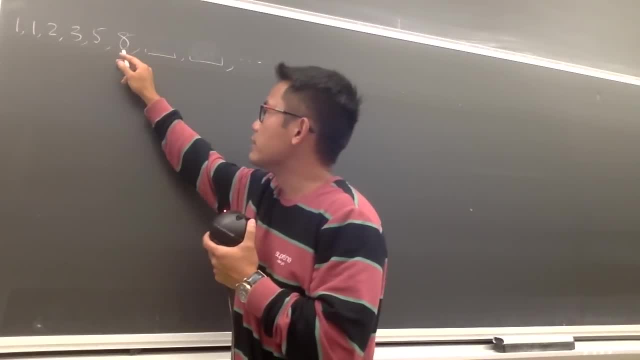 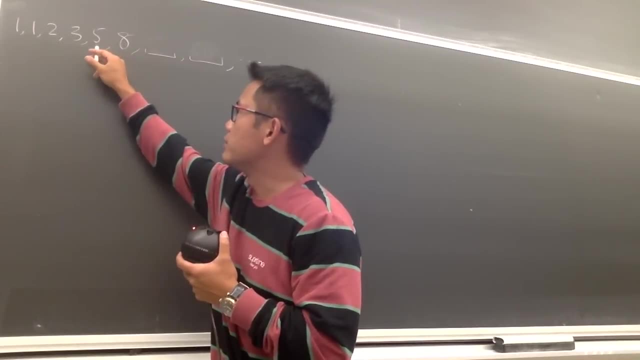 For example, how can we figure out this term? Well, let's look at 8 first. You know, 8 is the same as 3 plus 5, right? And to figure this out, it's the same as the sum of the previous two terms. 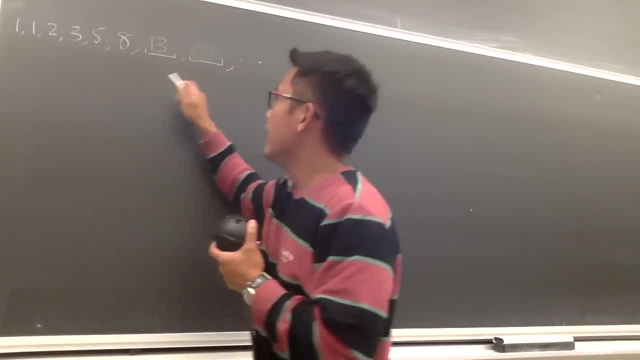 So to do this, we just do 5 plus 8,, which is going to be 13.. And likewise for this term, we just have to do 8 plus 13,, and that's going to give us 21,, right?